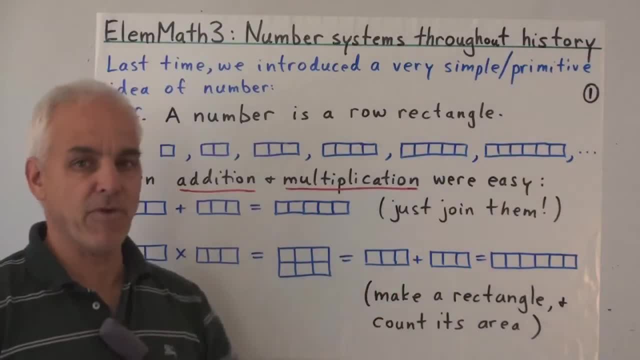 And so on. So we haven't actually given these numbers any names so far. The lovely thing about thinking about numbers so naively is that addition and multiplication are conceptually very easy. If we have two numbers like 1, 1 and 1, 1, 1, then to add them we just put the two rectangles together, We just join them up. 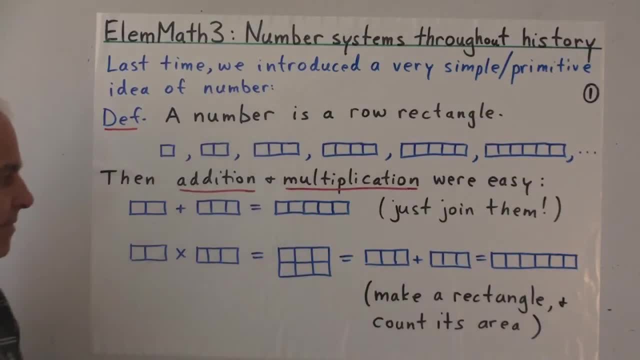 So the result is 1, 1, 1, 1.. Which of course we would say as 2 plus 3 equals 5.. But we haven't given these numbers their normal names yet. Multiplication is not much harder. So 2 times 3, or 1, 1 times 1, 1, 1 in our primitive language is defined as what you get when you count the number of cells in this rectangle. 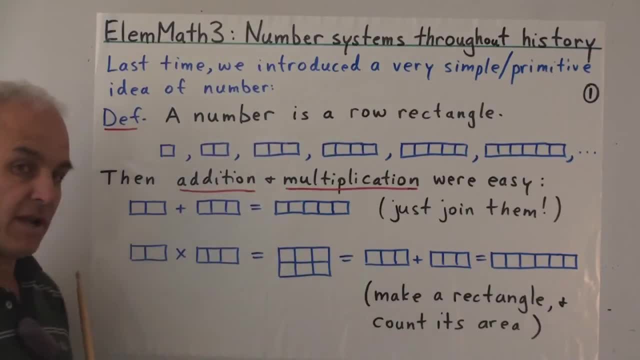 The rectangle which has the same number of rows as our first number and the same number of columns as our second number. So two rows, three columns. It's a two by three rectangle, using our earlier convention for dimensions of a rectangle. So we have to count the number of cells here and one. 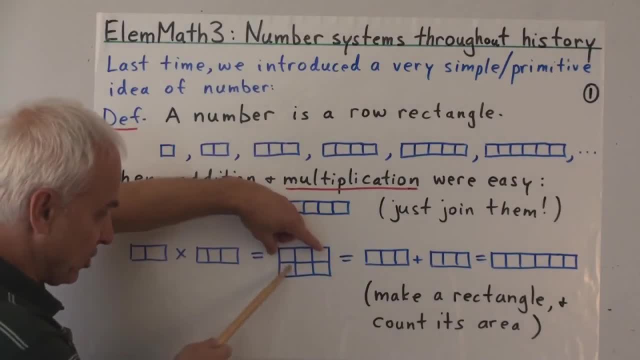 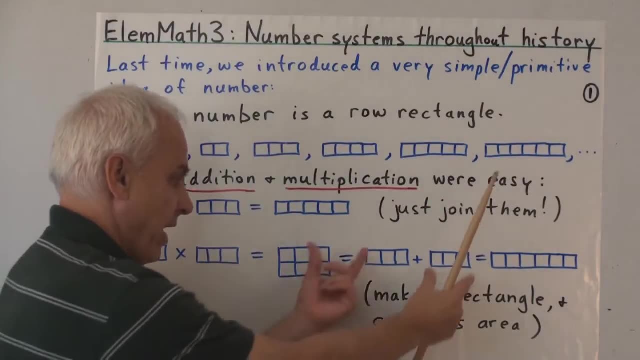 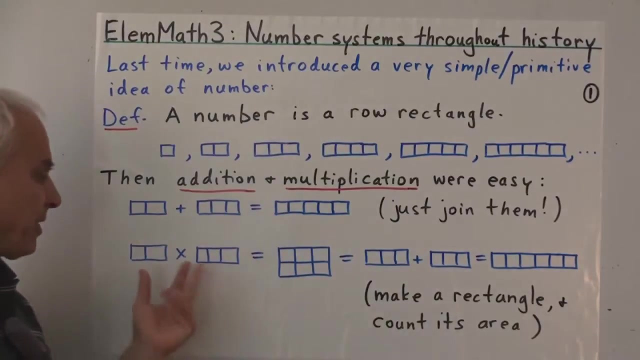 way of thinking about that is just to divide this rectangle up into its two rows and put the rows one after the other- First row followed by the second row- and add them by putting them together. What this shows is that another way of thinking about what the multiplication means is that we're 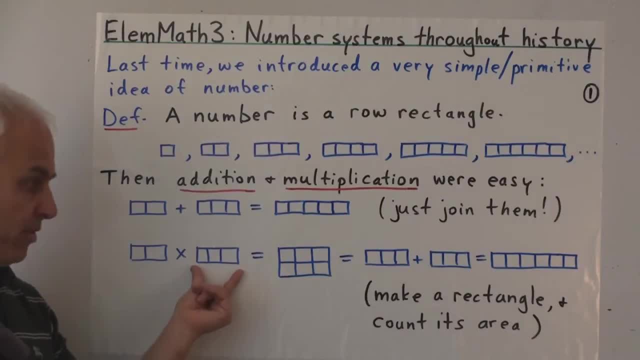 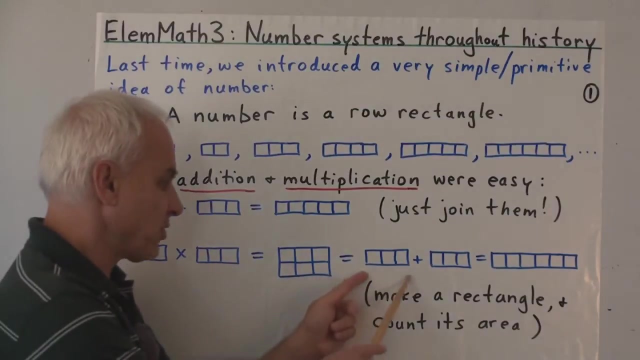 taking copies of this second number, the three, and how many copies are we taking? We're taking one copy for each of the cells in the first number, So we're really taking two copies of three. There's the first copy of three. there's. 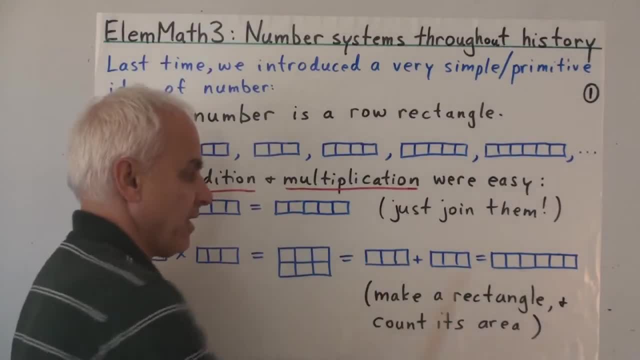 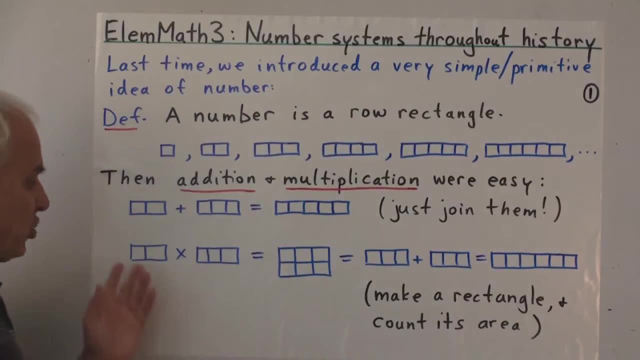 the second copy of three And adding them together to get the answer. So these two ways of thinking about multiplication are equivalent. We can think of two times three as being two copies of three added together, or we can think of the number of cells in this. 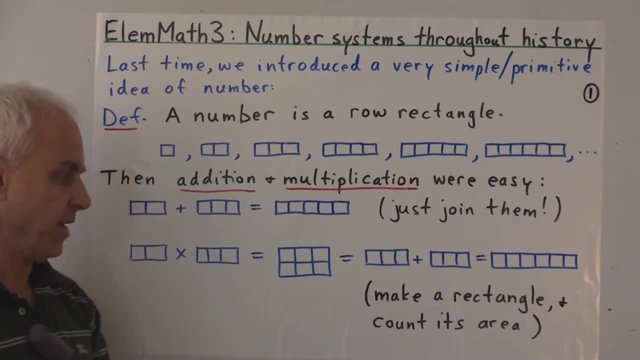 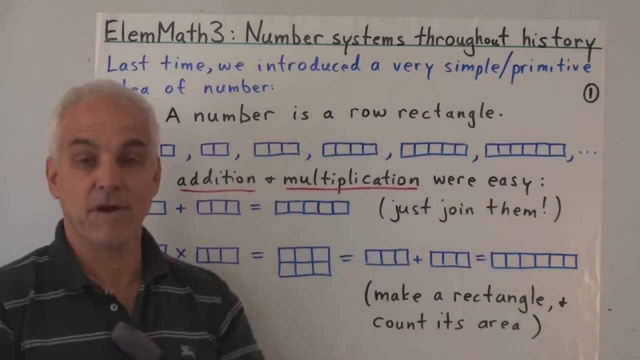 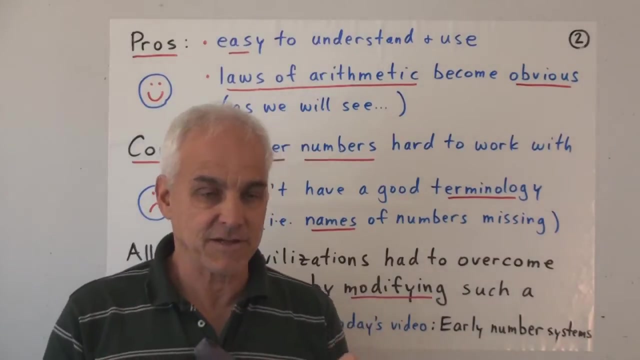 rectangle whose dimensions are two and three. Okay, so that's addition and multiplication, defined using this very naive notion of number. There are some obvious pros and cons to working with such a naive system. The pros are that, first of all, it's easy to understand and pretty easy. 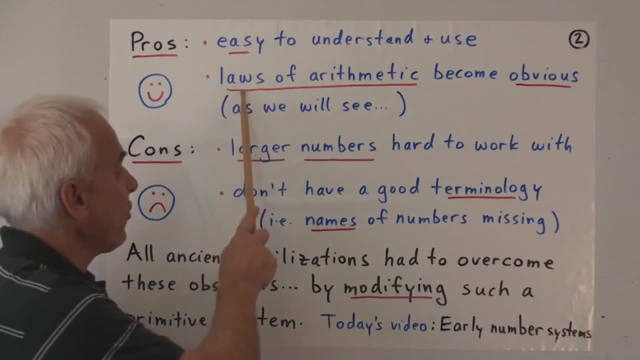 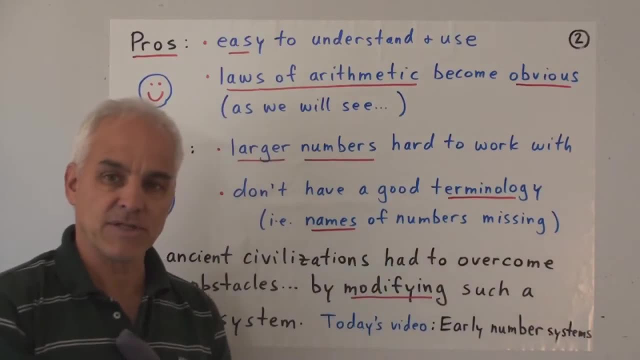 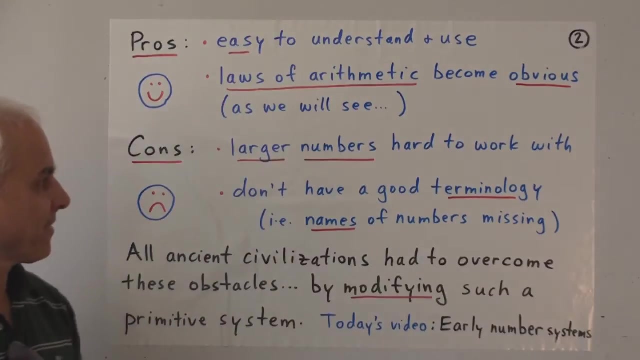 to use. Furthermore, the laws of arithmetic, as we'll see, eventually become very simple to understand. They become almost obvious when we present them in this direct geometrical way. What about the cons of this point of view? Well, first of all, larger numbers. 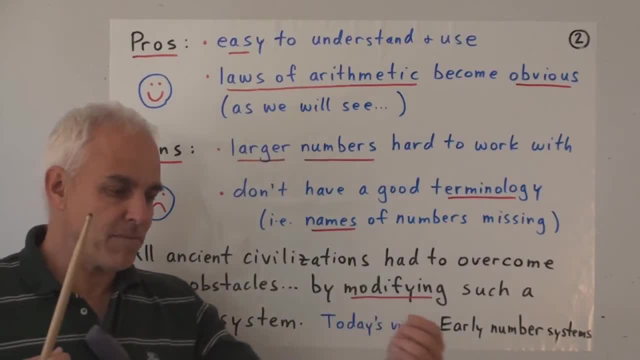 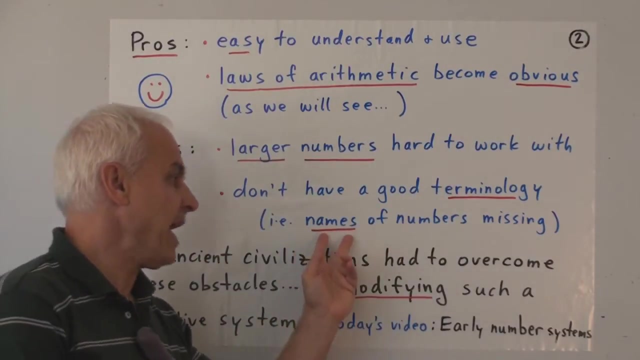 are clearly hard to work with. Once we get past 10,, 20,, 30,, we're having such long strings that it's painful to write all those little squares. And secondly, we don't have a good terminology yet we don't have good names for the numbers. 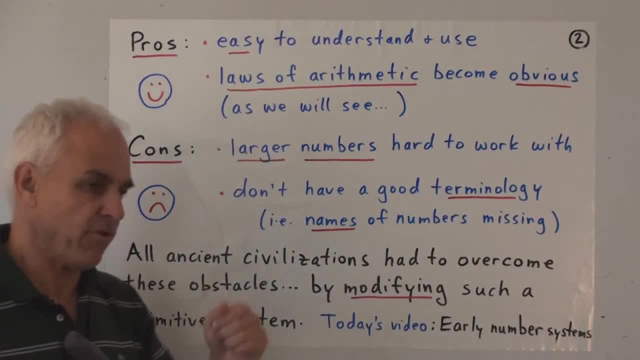 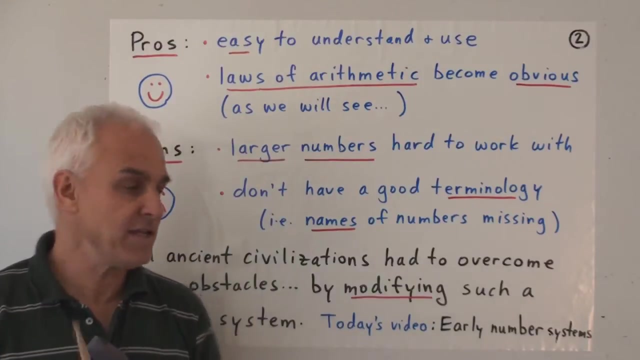 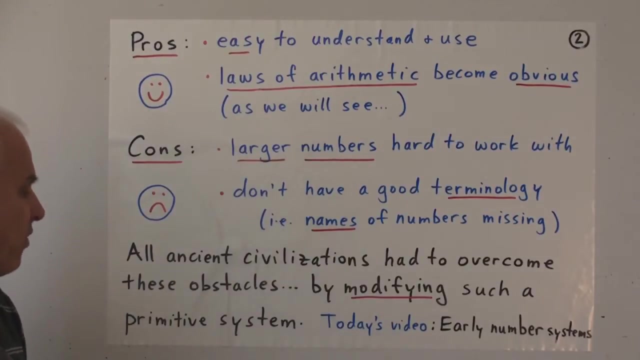 Calling numbers one-one-one-one-one-one-one is clearly of rather limited use. All right, all ancient civilizations had to overcome these kind of obstacles, and all ancient civilizations had to find ways of dealing with larger numbers and introducing some kind of terminology and notation for them. So in today's video we're going to look at some of these. 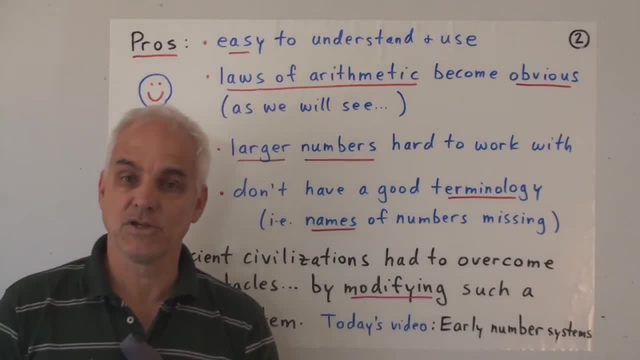 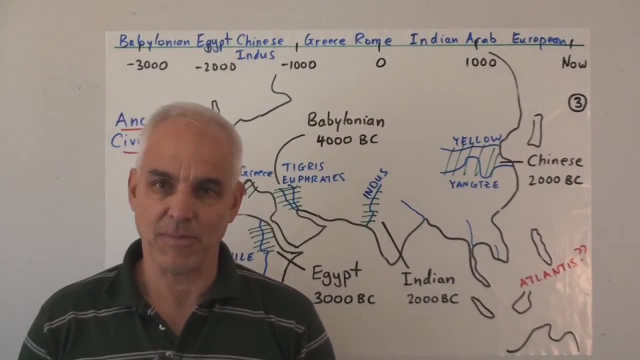 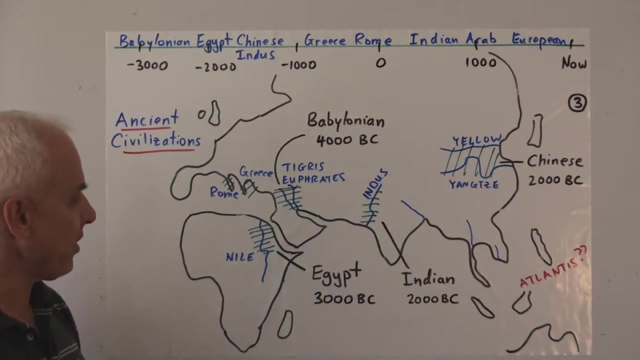 early number systems that arose in different parts of the ancient world. Let's have a brief look at some ancient civilizations. Just touch a little bit on some history. Here is a map of a good part of the world and on it I've drawn where various important ancient civilizations started. So we have ancient 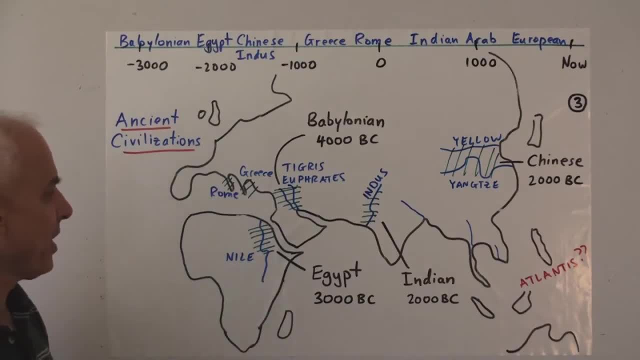 Egypt along the Nile Valley in Africa. We have ancient Mesopotamia, or sometimes called the Babylonian period. In the Middle East, we have the Babylonian period In the Middle East. we have the Babylonian period In the Middle East. we have the Babylonian period In the Middle East. 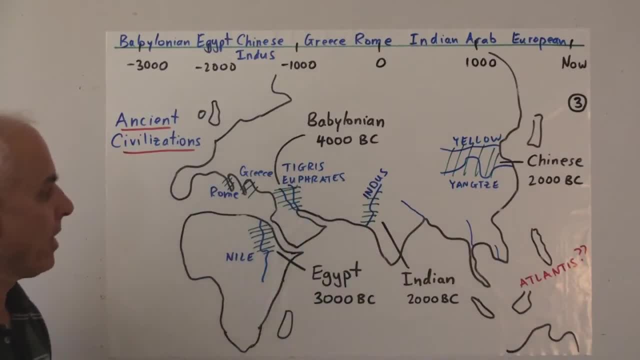 between the Tigris and Euphrates rivers. We have Indus civilization on the Indus river between Pakistan and India. We have Chinese civilization between Yellow and Yangtze rivers with, very roughly, these kind of dates: 2000,, 2000,, 4000, 3000.. So in our calendar here, which is a linear representation of the time, 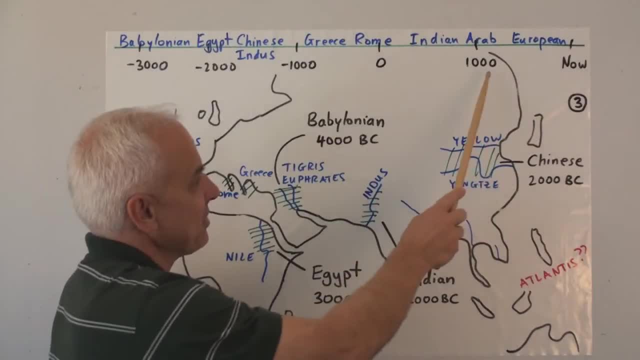 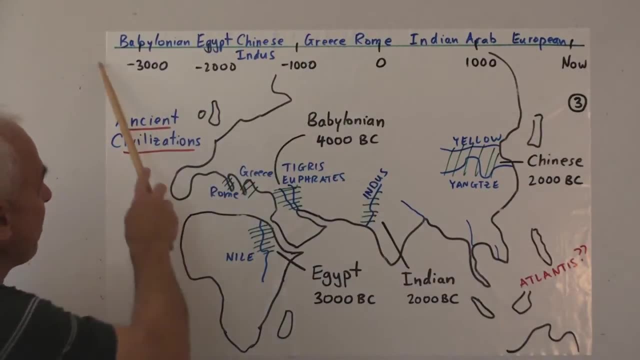 so here's now roughly the year 2000, then here the year 1000, year 0,, 1000 BC, 2000 BC, 3000 BC. So the Babylonian period would have been starting around here and the Egyptian period more or less concurrently, maybe a little bit shortly. 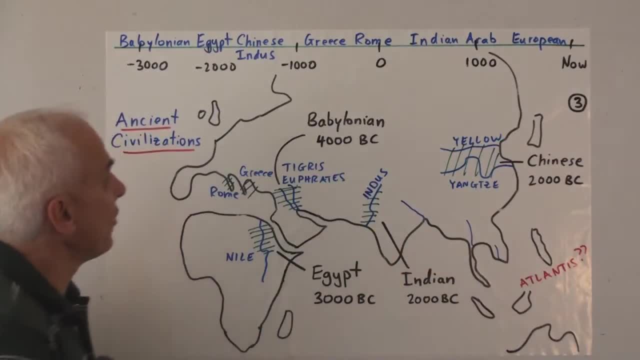 after, And then the Chinese and Indus sort of in this region here around year 2000 BC. Later on, of course, civilizations came and went And eventually Greece here in Europe became important, So that's sort of around 1000 BC to 500, 300 BC. And then Rome picked up sort of after that eventually had a big 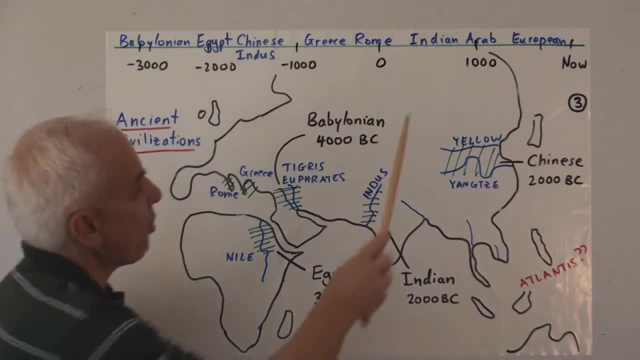 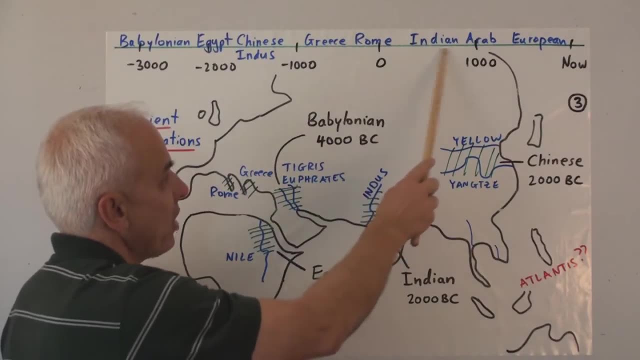 empire Mathematically. later, there was a very important period where other Indian mathematicians not necessarily centered around Indus Valley, but other Indian mathematicians made important contributions in the years 500 to 1000 or 1200. And also around this time the 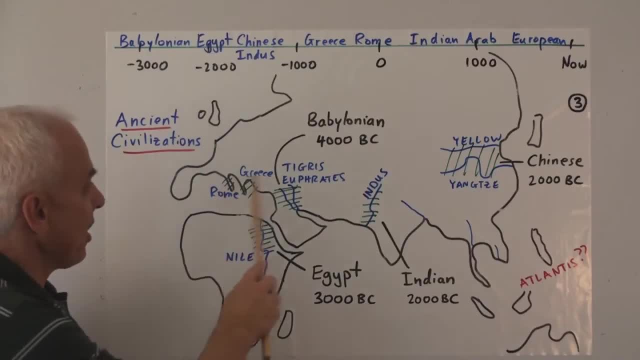 Arabs or the Persian peoples, carved out a big empire and became very scientifically sort of capable and assumed a leading role, And then finally more in the European setting around the middle of the last millennium, around 1400 or so. then Europe started to develop and take the lead scientifically Alright. so today we're going to look at these. 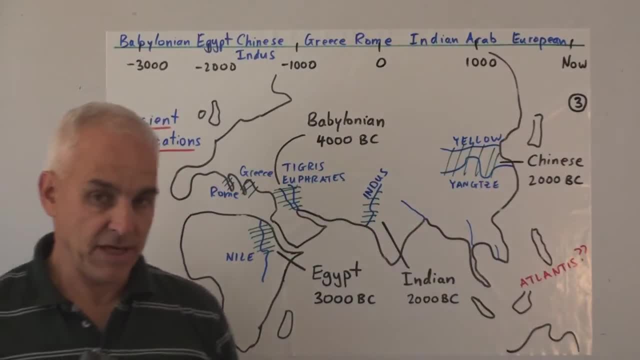 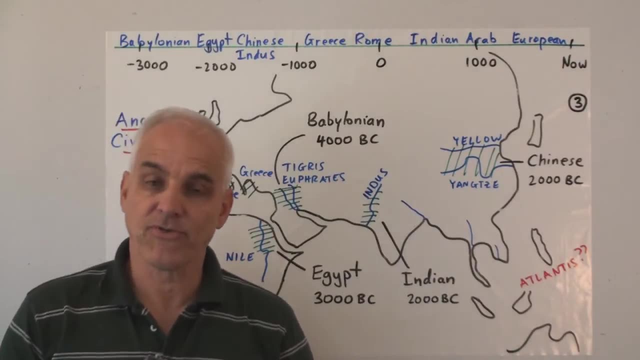 ancient civilizations and we're interested in the question of how they, how they developed a number system to do commerce, to do calendar reckoning, to take care of large-scale agriculture, which would have been the main activity of these cultures, to deal with various issues of, you know, population armies. 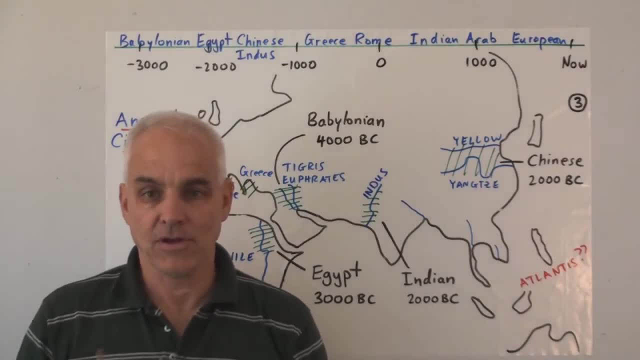 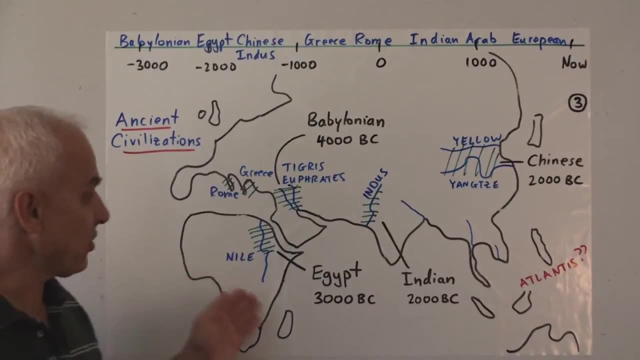 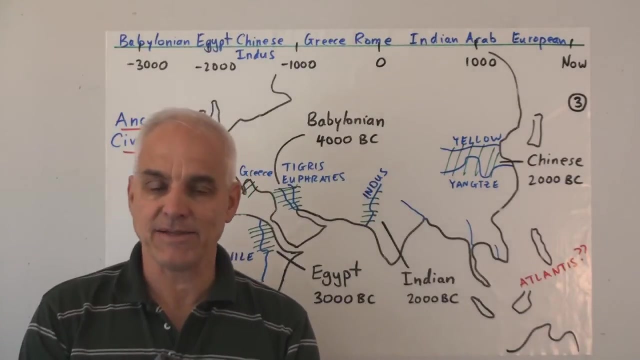 prisoners and so on, and how to organize large states requires some obvious facility with basic arithmetic. So they would have had a number system and it's sort of interesting to have a look at various ones. Before we do that, let's try it ourselves. Let's go back and see what would we do if we had to start off on 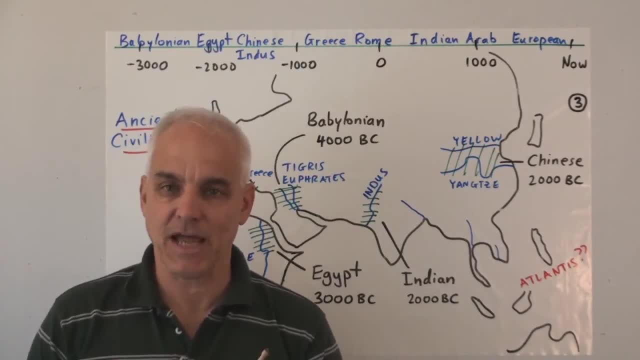 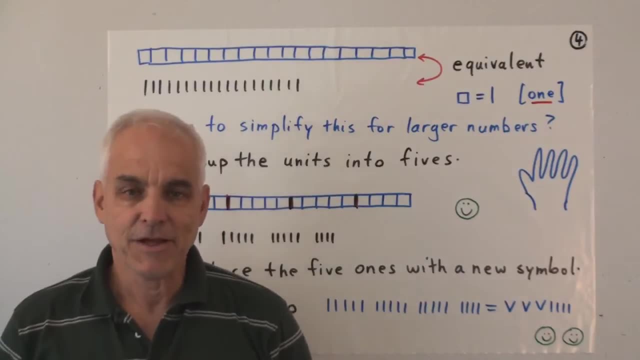 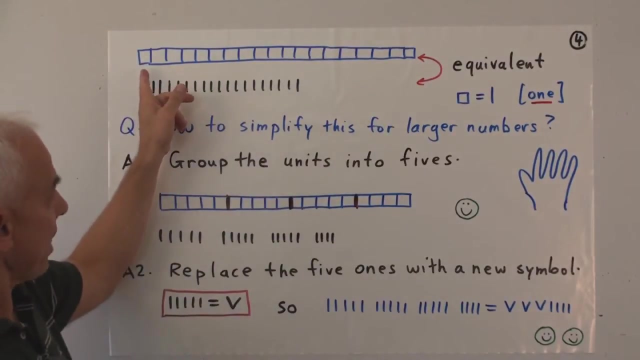 our own to develop a number system which is a little bit more sophisticated than just making a lot of strokes on a page. So I told you that mathematics is really just common sense. So how would you deal with this problem? Suppose you had to work with numbers and at this point numbers are long. 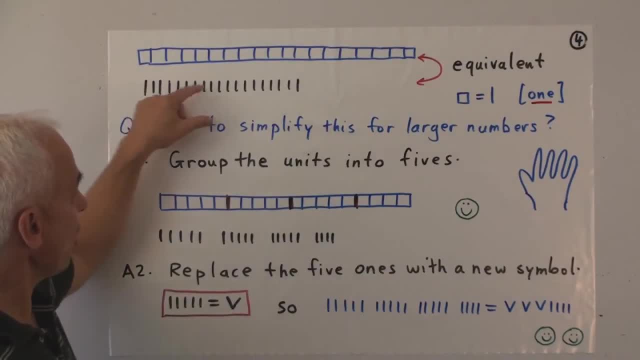 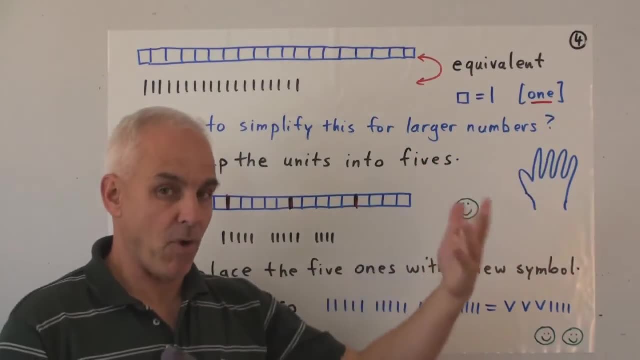 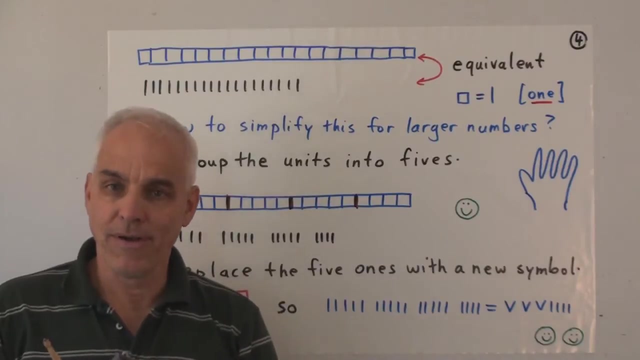 rectangles or maybe equivalently long strings of strokes on a page. So whether we think about little squares, whether we think about strokes on the page, they both represent the number one. it's more or less equivalent, And it's clear this is going to be unwieldy for larger numbers. So what are you going to do to? 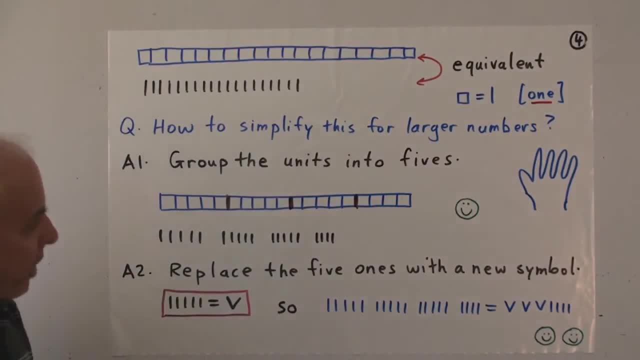 deal with larger numbers. Well, I think most people would come to something like this. They would say: all right, well, let's take a big number, whether it's a long rectangle or whether it's a string of strokes, and let's subdivide it into some. 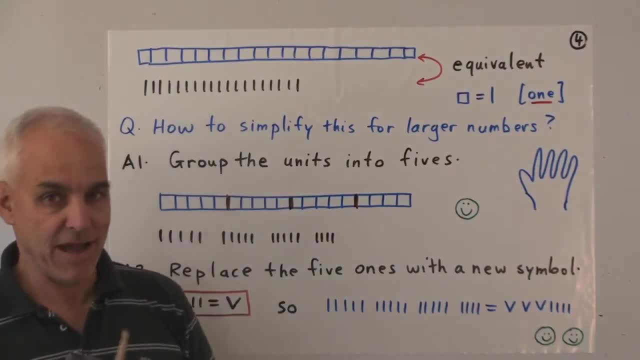 useful unit And five is a pretty number And five is a pretty number And five is a pretty number And five is a natural unit because we have five fingers on our hand. So it would be very instructive to split a long rectangle like this into parts with five units. 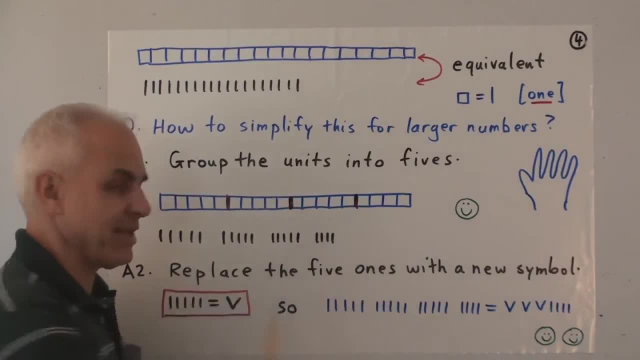 each Five, five, five, and then whatever is left over once we get to the end In terms of a string of strokes. well, we could do the same thing by sort of making a little bit of a separation: Separate that five from that five from. 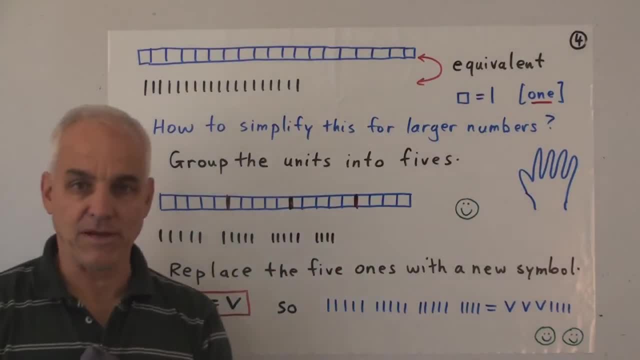 that five and then from the rest and then becomes much simpler to read. So this is already a big advance to creating a little some gaps or some some delineations to structure our long number. The next step would be to think: well, all right, we've got these units of five, Why do we need to keep on? 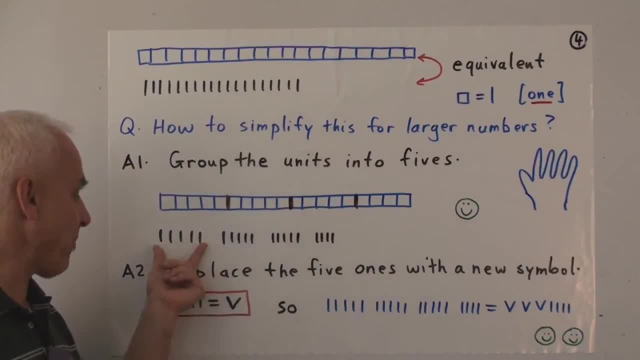 repeating them. then If we know this is going to be five, we can represent this group of five by some new symbol. And why don't we represent five with the symbol V? That's reasonably natural, because if you have five fingers like this and you look at the hand, you kind of see a V, So V looks. 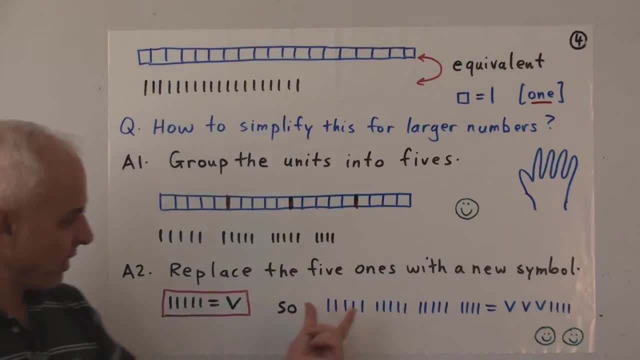 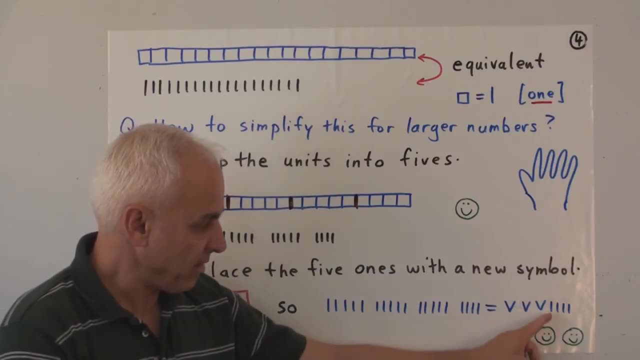 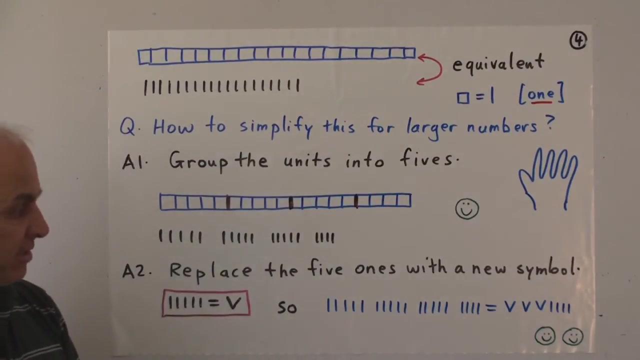 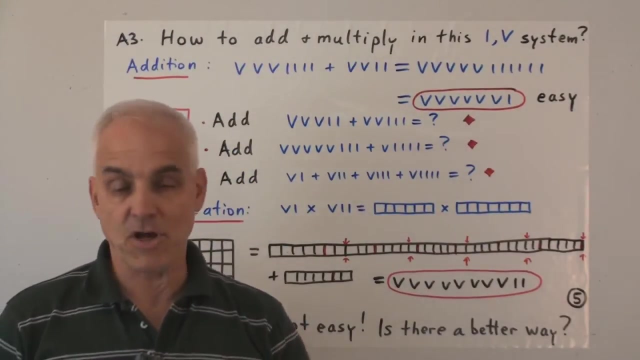 like a hand. So this number here, which we would have written with five, five, five and then four, we can now write with the symbol VVV1111.. And we've simplified our number reasonably well. We're happy. So the next natural question is: well, how do our basic 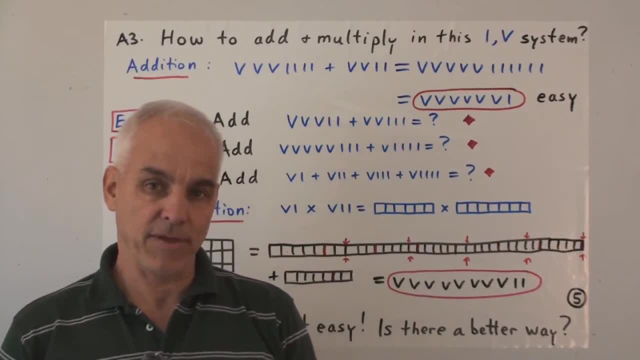 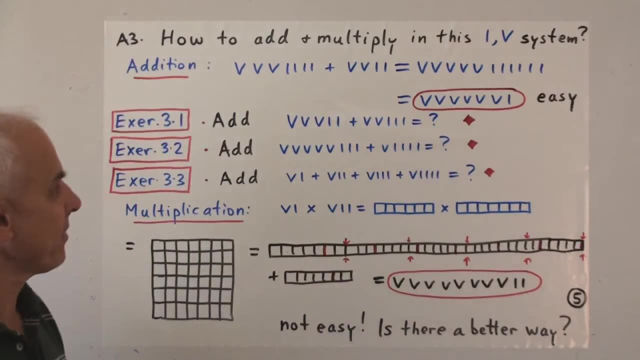 operations of addition and multiplication work with this new system where we have not just ones but also V's or fives. Well, let's say, we want to add this number and this number now with V's and ones: VVV1111 plus VV11.. 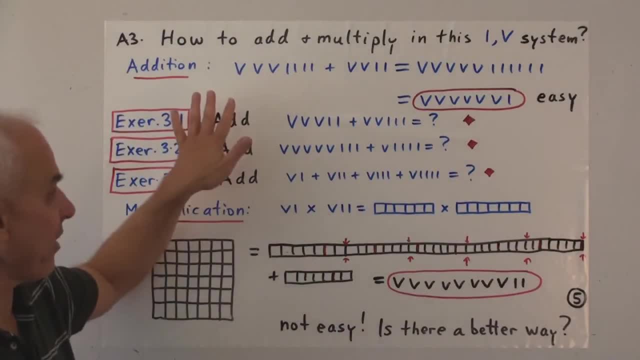 Well, each of these V's represents a group of five. So there's a group of five, There's another group of five, Another group of five, There's one more, There's one more. When we combine them all, we're still. 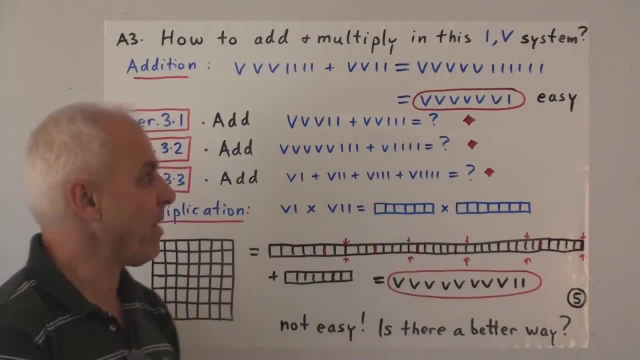 thinking of our string of ones in the back of our minds. So a moment's thought shows that we can combine this in the simplest possible way, just by bringing all the V's here and all the V's here together. So there were three V's here. 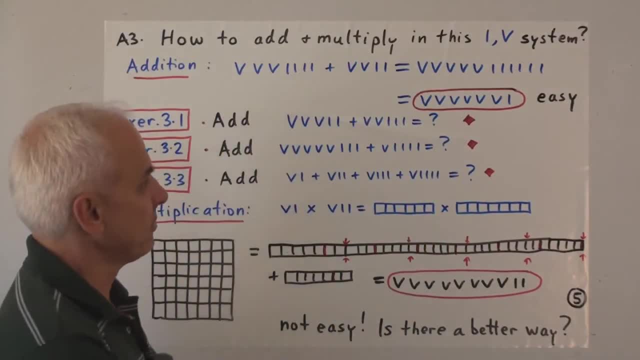 and two V's here. Now we've put all of them together up at the front And the number four ones here and two ones, And we've strung those at the back. Now when we look at this for a second, we say, well, wait a minute, that's interesting Here. 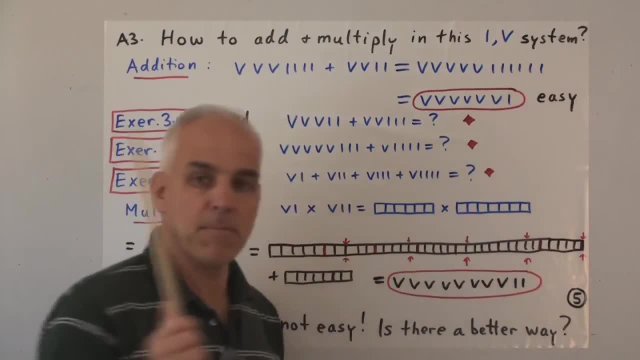 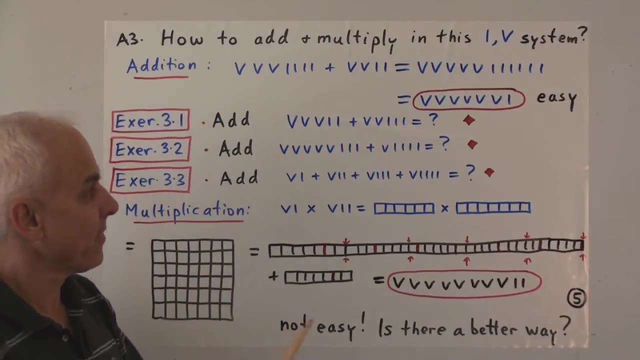 how many ones do we have? We have one, two, three, four, five ones. We can simplify that a little bit because we've said that those five ones can be replaced with a V. So we'll keep all of these V's that we had before and we'll add one. 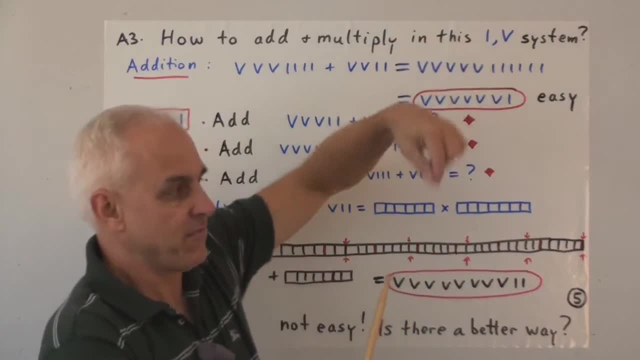 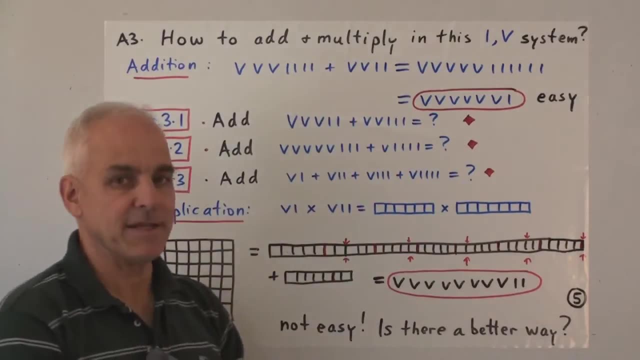 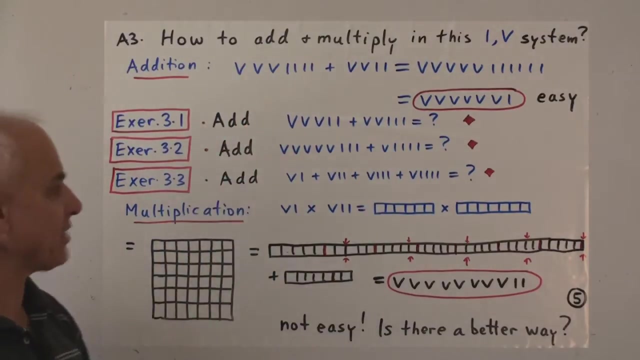 more V, Meaning that we don't need to put in those five ones, But there still will be that one left over. So that's reasonably easy to do addition in this sort of new system. Okay, here are three little exercises for you to make some computations of addition in this system. So you're not 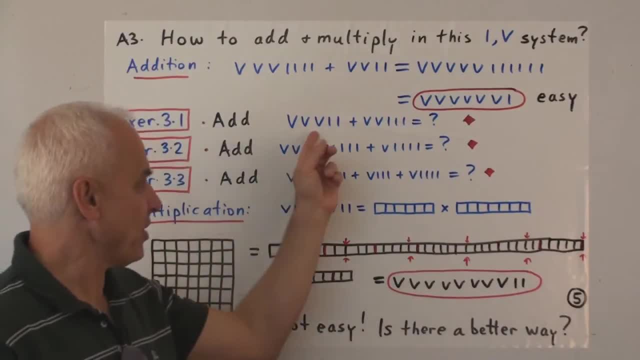 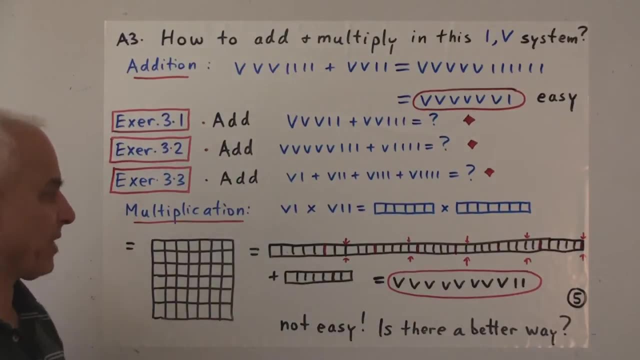 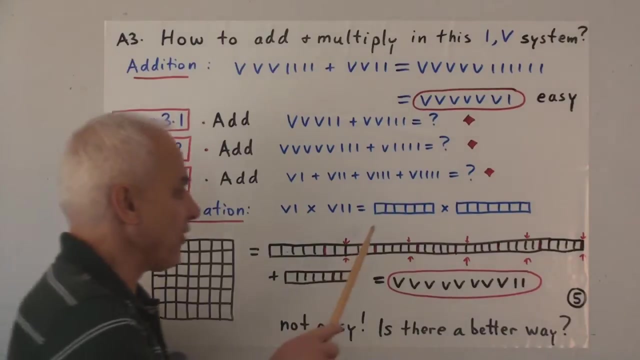 allowed to convert it to ordinary numbers and then do the arithmetic. I just want you to work in this system to figure out what the answers are. Well, how about multiplication? Suppose that we wanted to multiply six times seven. So I just remind you that here's our rectangle for six and here's our 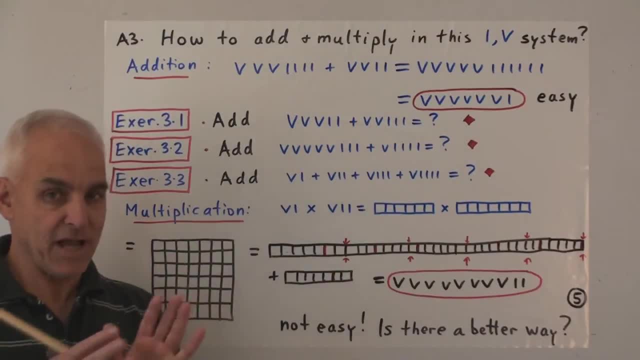 rectangle for seven, And we saw that multiplication is nice when you think in terms of rectangles. You can make a new rectangle with six rows and seven columns And then you count how many cells it has. That's the answer. So you can count how many cells it has by taking each of these. 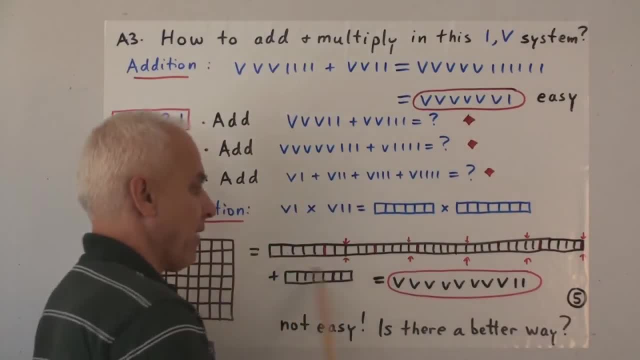 rows and stringing them up there. I ran out of space here so I couldn't keep going, so I took the liberty of adding the rest. So I claim that in here, together with this, there's as many cells as there are right here. So this cumulative thing is the number. 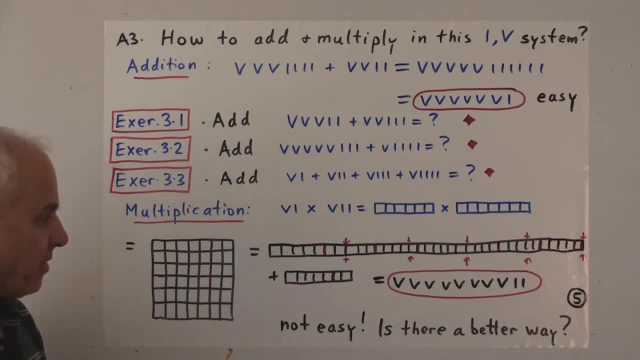 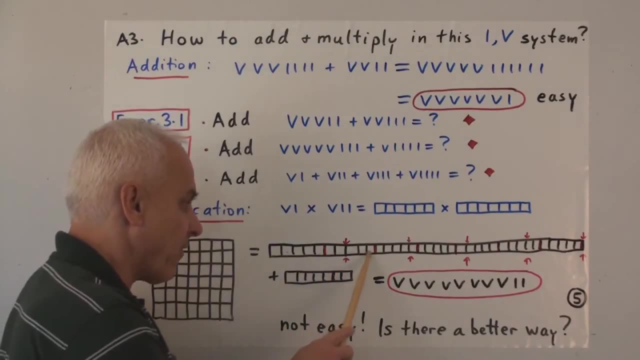 Okay, now what we do is we want to convert that by breaking it up into fives. So the red here signifies that first five, One, two, three, four, five, There's another five, There's another five, Another five, Another. 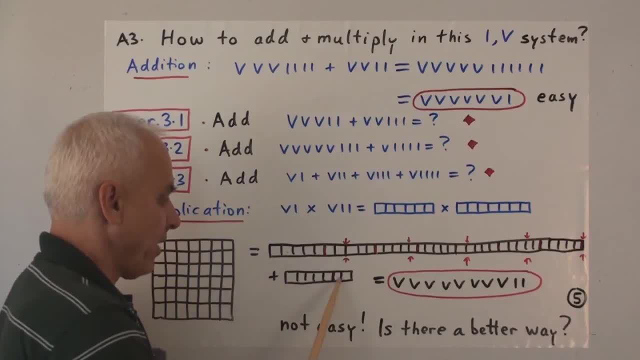 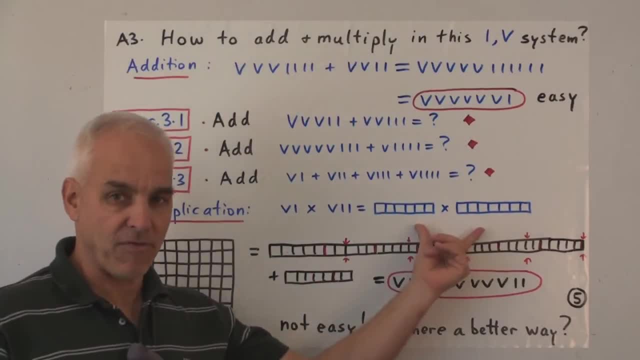 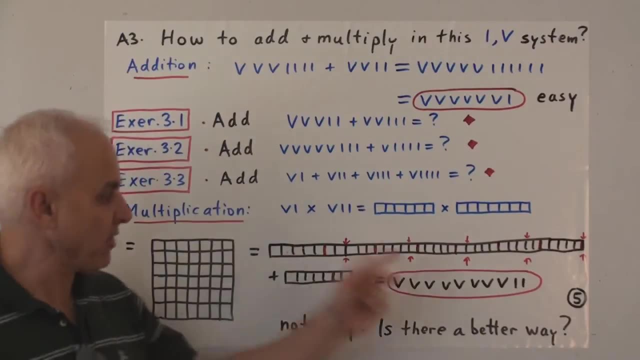 one V form, converted them back to our more primitive idea of a rectangle, made the computation with the rectangles and then at the end converted back. If you did this a lot, with lots of examples, you would probably start asking yourself: well, can I just go from here to here without 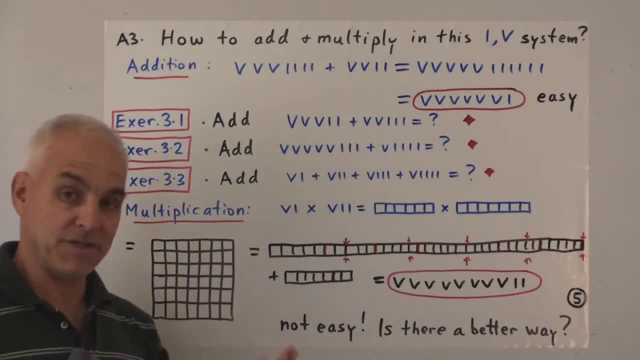 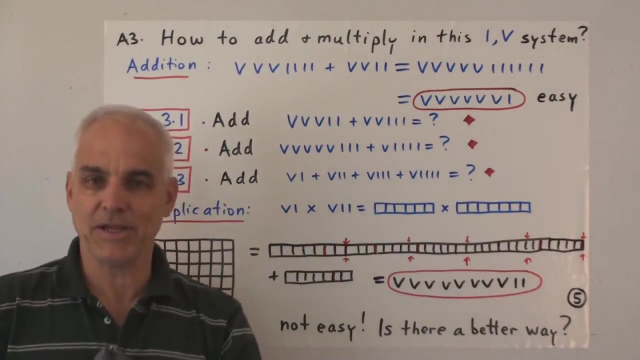 having to do all this rectangle business. Are there some simple rules that let me know when I multiply two numbers directly? Well, that's a very good question, And there are such rules, but they're not entirely easy. They require some thought and some understanding. 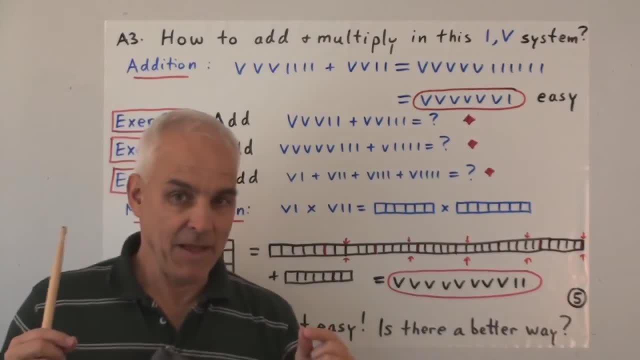 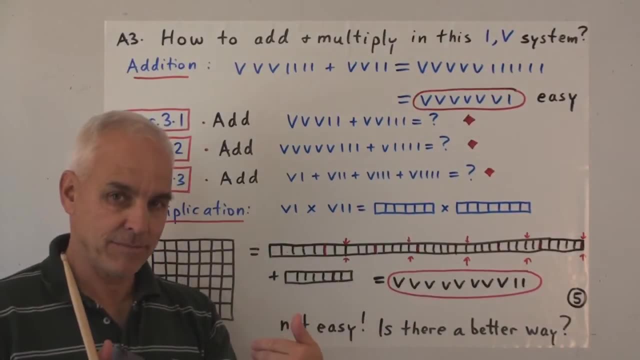 of what's going on. So already we see an important trade off here. Our notation is becoming more compact, but the rules for the operations become more complicated. That's kind of a trade off in this game. The more compact and efficient your notation, somehow the more complexity involved in doing the multiplication. 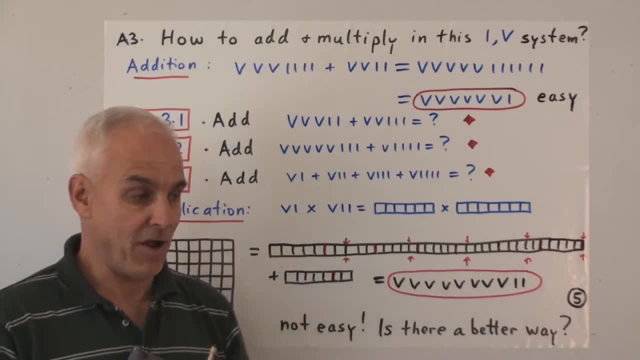 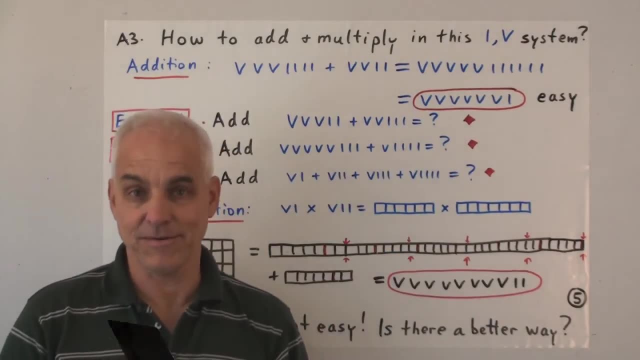 or operations generally. We'll see that as we carry on. So now let's have a look at ancient civilizations. What did they do? Did they do something like this? Well, yes, they did. So the first system that we'll look at is not the oldest, it's one of the newest, But 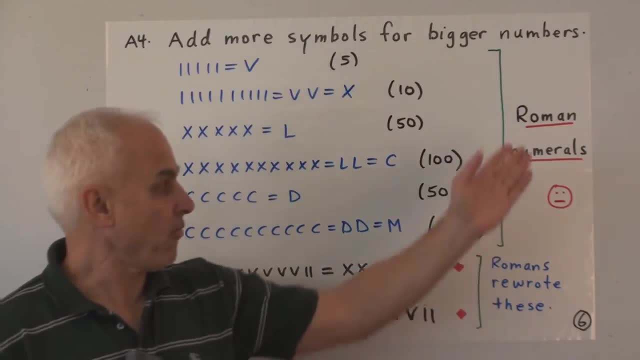 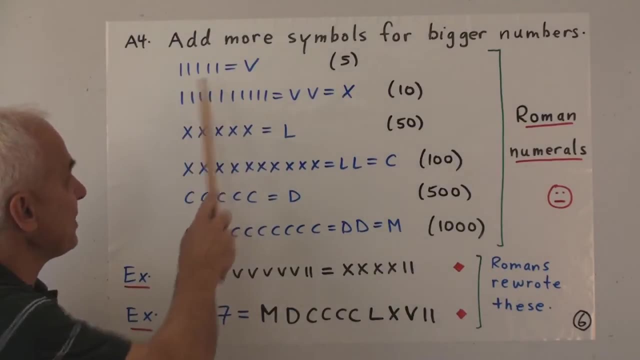 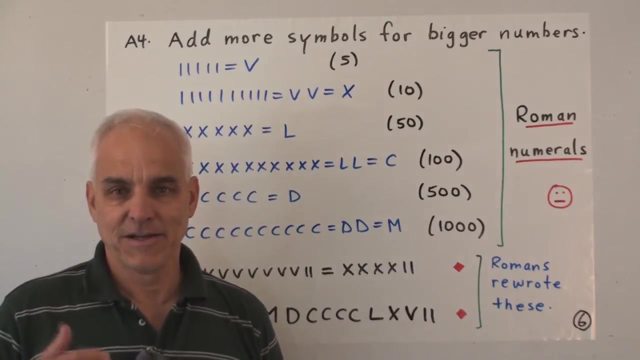 it's the one that's probably most familiar. It's the system for Roman numerals, And the Roman numerals start exactly as we've started, by replacing five strokes with the letter V. The next step is to add some more symbols for bigger numbers. We saw even in the previous example that we can get a lot of V's piling. 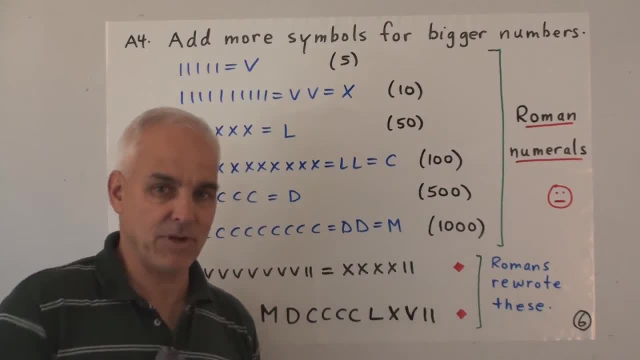 up. So just as we replaced ones with these, we'd like to replace V's with some other denomination. It's a lot like money, isn't it? We start off with one dollar coins or one dollar bills, And then, to make life simpler, we introduce a five. 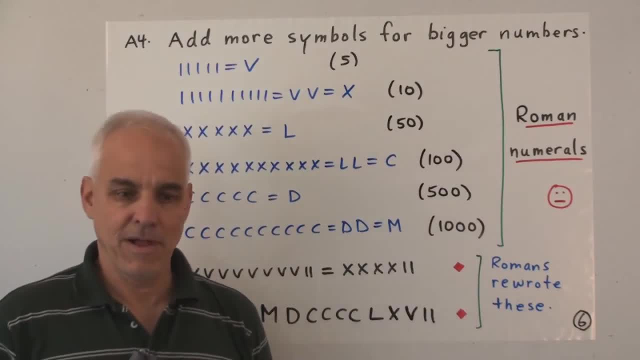 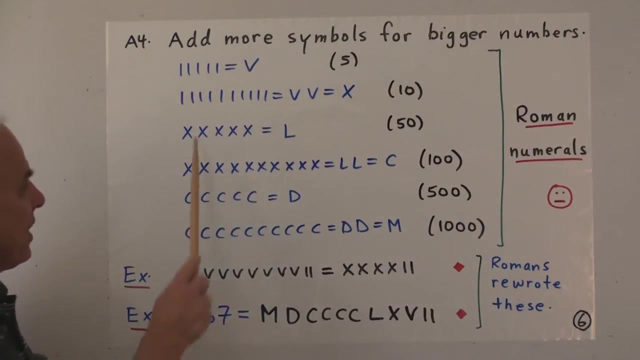 dollar bill and then a ten dollar bill, And the more commerce we're doing, the larger amounts of money we're working with, the bigger kind of denominations we need. So the Romans introduced a symbol for ten, That's X, So that's representing either ten ones in a row or two fives in a row. They also introduced 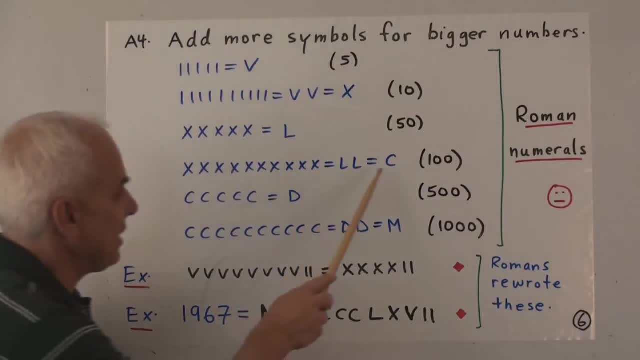 an L for fifty, A C for a hundred, So a hundred is ten tens, Or two fifties, A D for five hundred, So there's five hundreds, make a D And a symbol M for a thousand, A thousand being ten hundreds. 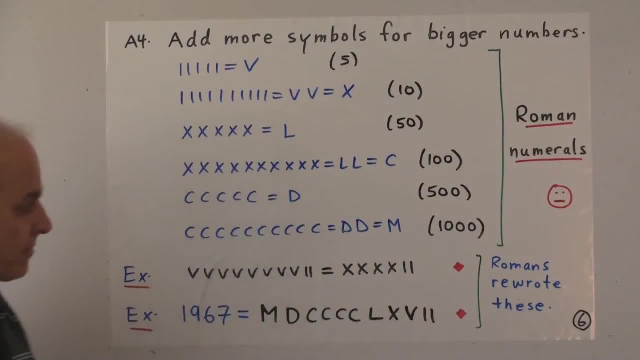 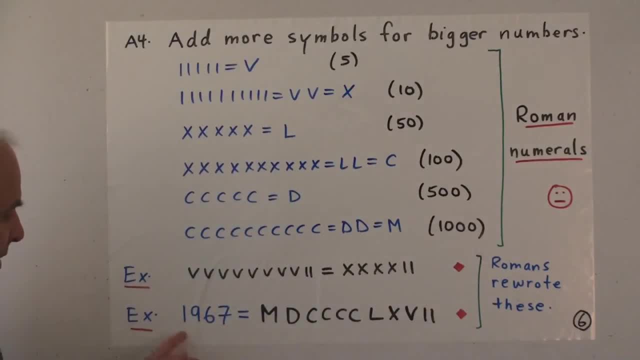 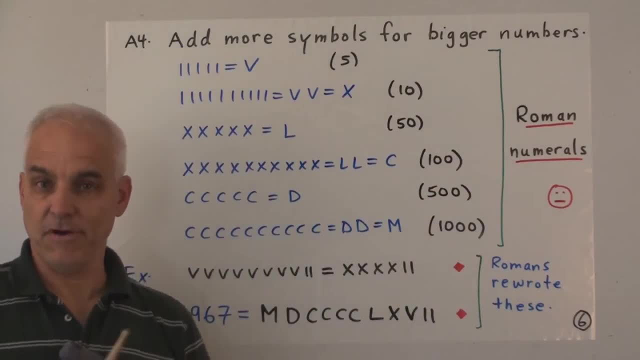 represents a thousand strokes. It's very efficient. A symbol M you should think of as replacing a thousand strokes. So we still have to replace these nine hundred and sixty-seven. Well, the next thing we would choose is a D, which represents five hundred strokes. Okay, we still need. 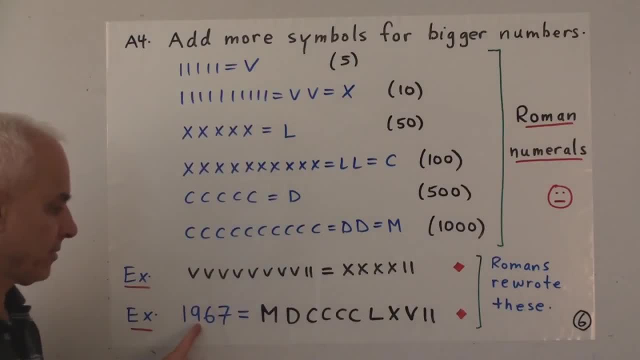 four more hundred. so we're going to put four C's together. So now we've taken care of a thousand strokes, and now here's another nine hundred. We still need sixty-seven more strokes to represent. How do we represent sixty? Well, with a fifty and a ten. So an L and an X, that would be sixty. And how do we represent seven? With a five and two ones. 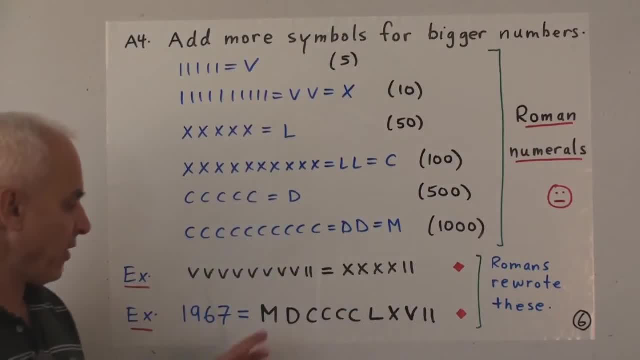 So this is a kind of a simplified way of writing nineteen, sixty-seven, Sixty-seven in Roman numerals. In fact, the Romans didn't write it exactly like this. They did some shortcuts, They introduced some extra little conventions that maybe I'll talk. 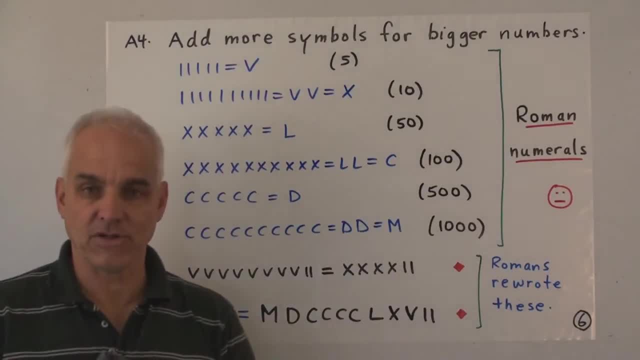 about at some point. maybe I won't, They're really mostly only of historical interest. Okay, so this was the number system that was used in Europe for a long time, until fourteen hundreds, fifteen hundreds, And it took a long while for the Europeans. 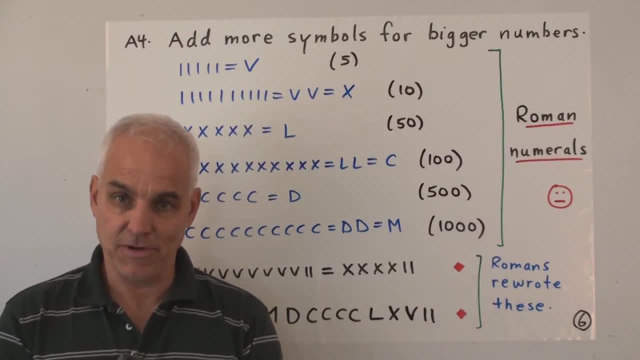 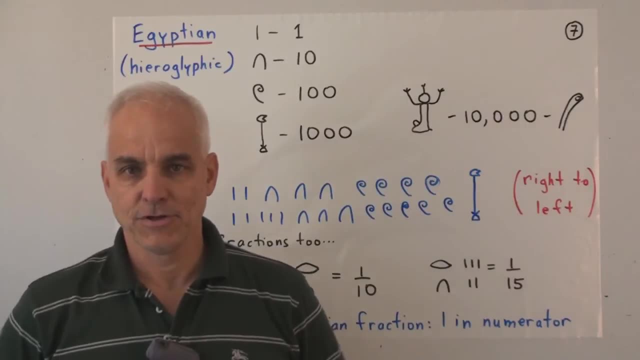 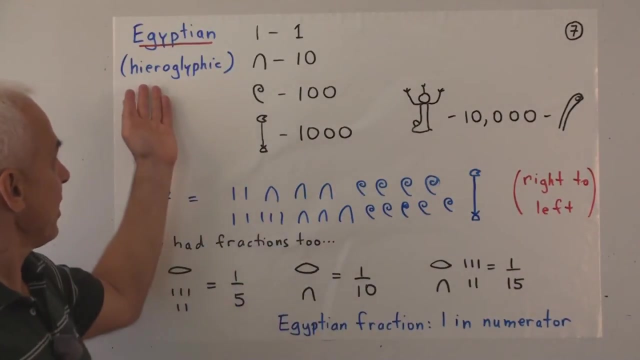 to finally figure out that the Hindu-Arabic number system was much superior than arithmetic with these Roman numerals. Now let's go back to ancient Egypt, to the land of the pyramids and mummies and temples. The Egyptians left us lots of inscriptions. 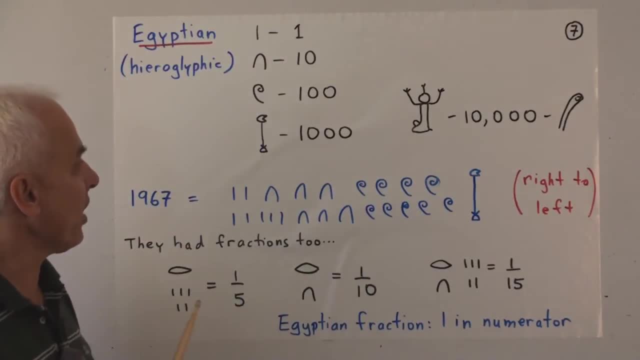 in their temples. so hieroglyphics and their number system is well understood. They had a system that's a little bit like the Roman ones, except that they didn't base it on five. They were a decimal-based system, So ten was the first unit that got a special symbol. 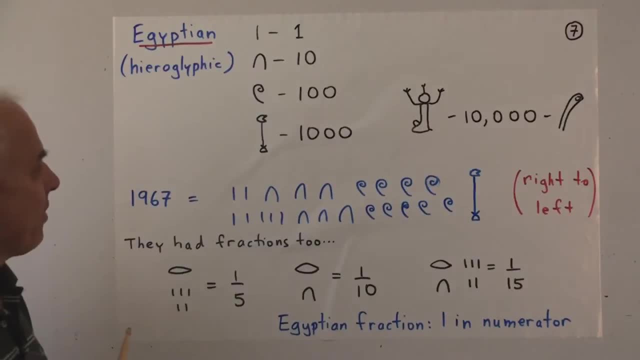 And this special symbol is this sort of upside-down U represented. ten Hundred is this little curly sign and the thousand is this long pole with something or other on it. My favorite is ten thousand. This has got to be one of the best numerical. 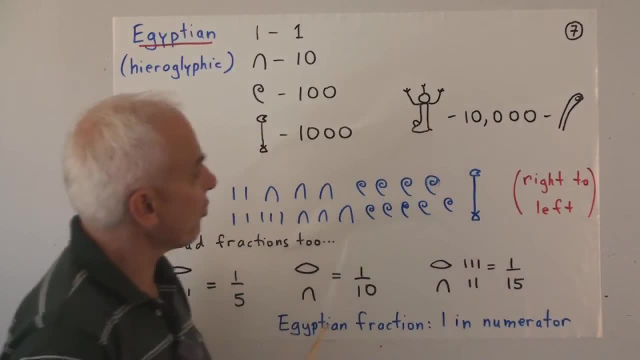 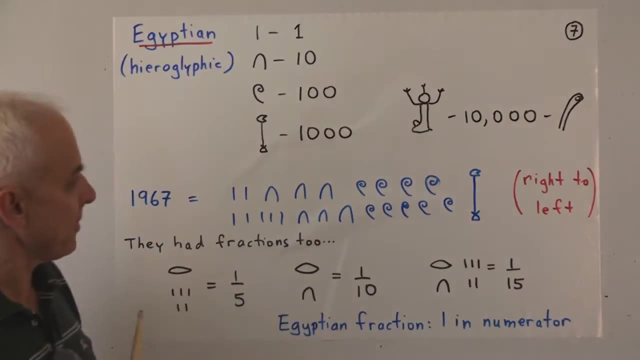 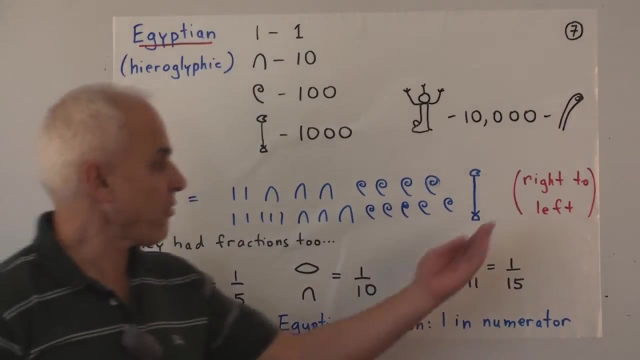 symbols of all time, this sort of kneeling person, praying or whatever, Although sometimes it's represented by a pointed finger, which is less interesting, I think. So how would the ancient Egyptians have written 1967?? Well, they read from right to left. 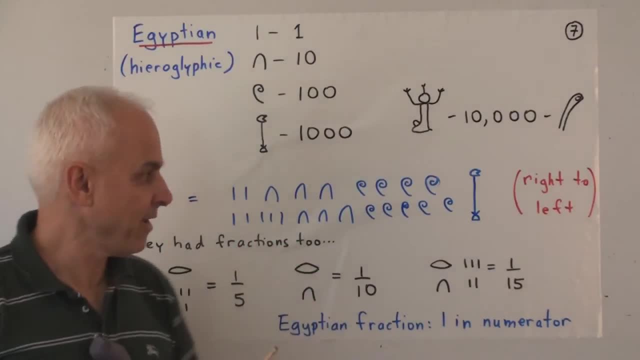 They still had the idea that we should deal with the biggest numbers first. So the biggest number is over here, That number, there is one thousand, That represents one thousand in there, And after that it's nine hundred, And indeed you can see nine of these curly 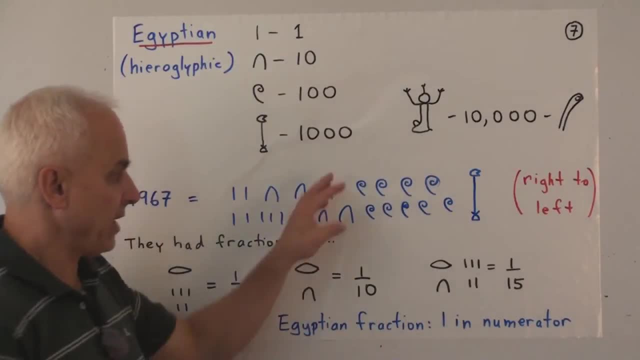 hundreds One, two, three, four, five, six, seven, eight, nine. They allowed themselves to use sort of two lines to put them in, And then after that we need to express sixty. Well, sixty is six. of those tens, There's one, two, three, four, five, six, And then 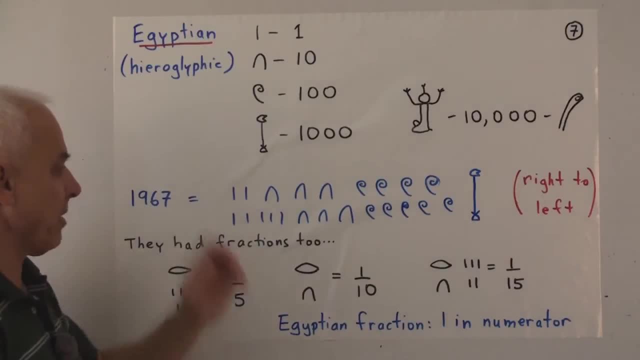 seven. well, it's just seven ones. We're allowed to put them on top of each other. It's worth mentioning that the Egyptians also had symbols for fractions. This sort of eye shaped here denoted to them a fraction. So this eye with a five underneath it represented one-fifth. An eye with a ten. 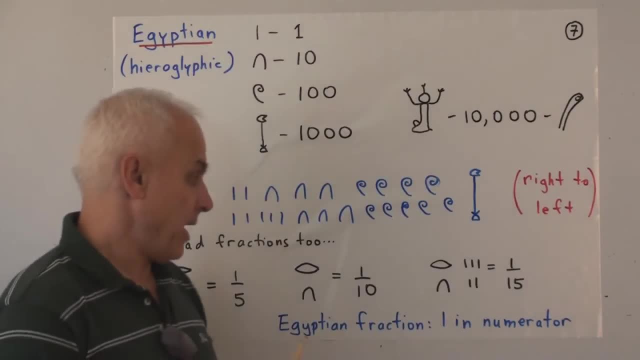 underneath it represented one-tenth And an eye. well, here there's a ten and a five, also sort of together there, So that's 15.. So that's one-fifteenth. You might ask, how would they have done three tenths? Well, curiously, the Egyptians didn't like. 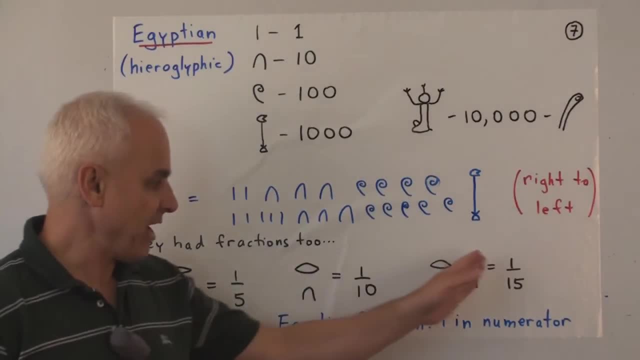 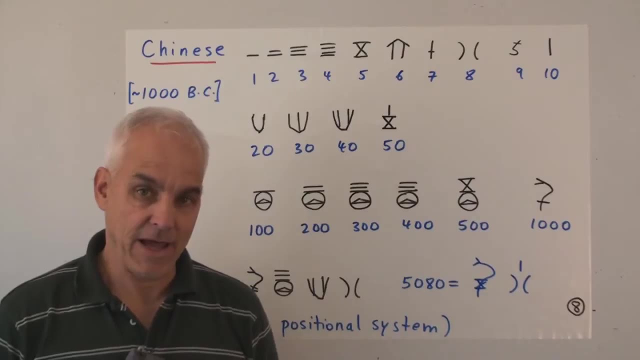 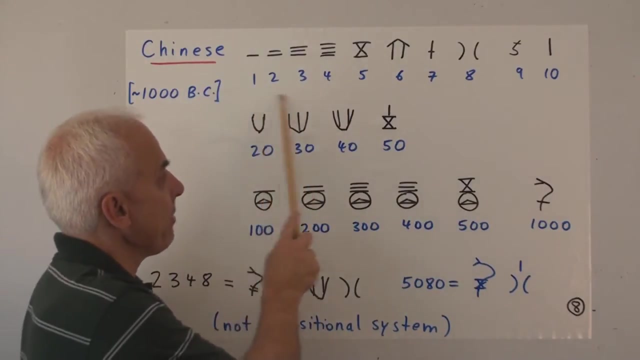 things like three tenths. They always tried to make their fractions have numerator one. These are sometimes called Egyptian fractions today. The ancient Chinese had a somewhat different system. They in fact had a separate notation for each of the numbers that we call, one through nine, even ten. So the symbol for 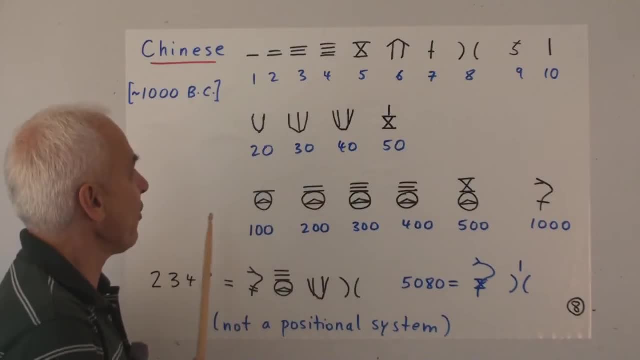 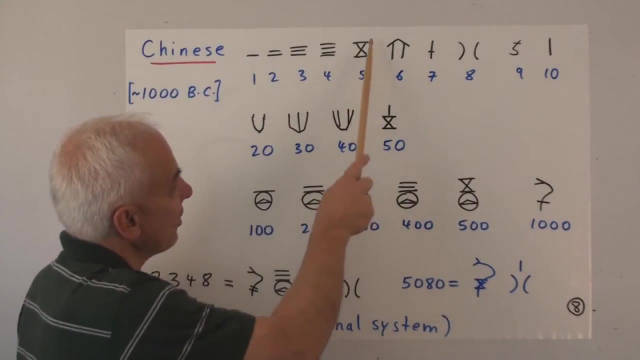 one is a lot like our stroke, except it's horizontal instead of vertical, and two and three and four are also pretty obviously the same kind of idea. But then five is this particular symbol, and then they had a separate symbol for six a. 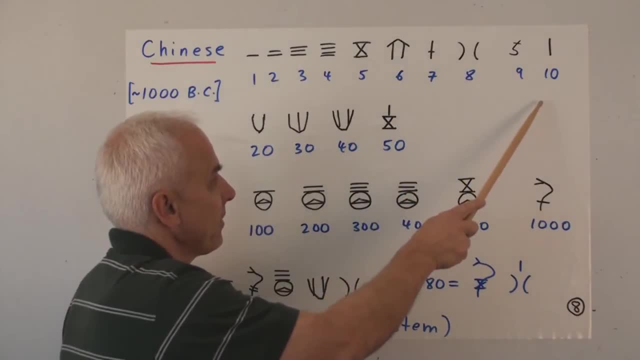 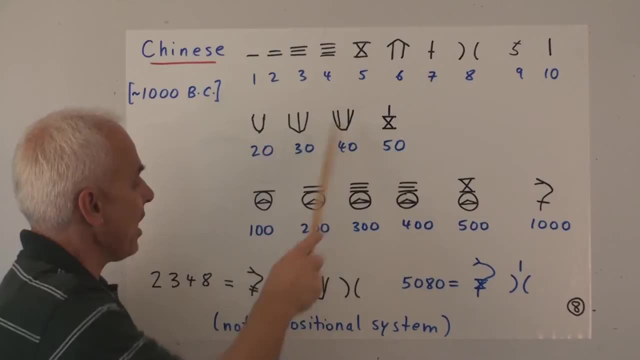 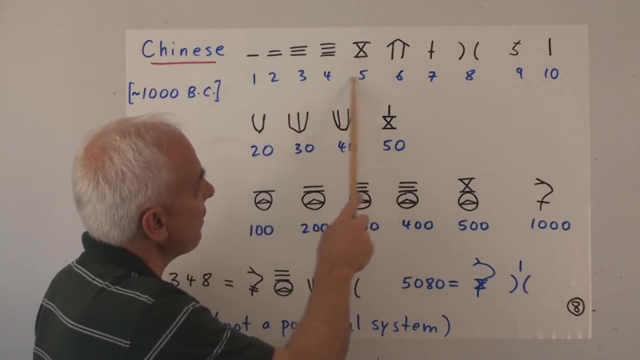 separate symbol for seven and for eight and for nine. Ten was just a straight bar. Well, twenty and thirty and forty were then some some kind of cup with the various lines on it. Then fifty was something like this: It's some kind of combination of five and ten. It's a kind of a multiplicative. 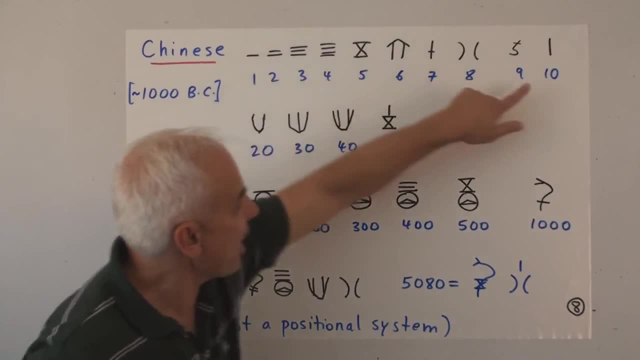 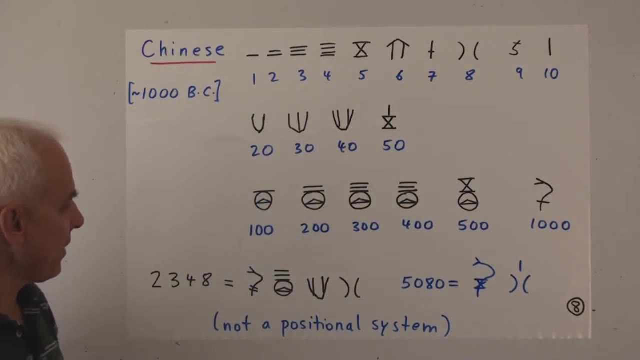 system, so that that one there is formed by taking five times ten. So we're combining the symbols for five and ten to get the symbol for fifty. There's a symbol for a hundred, and the symbol for two hundred is a symbol for one hundred. 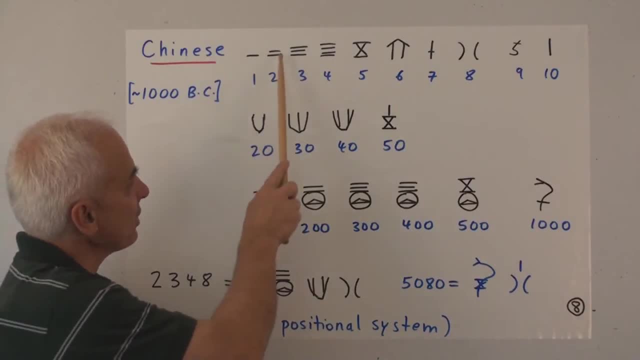 with two bars on top of it, So sort of we're multiplying the two by a hundred, and there for three hundred, for four hundred and for five hundred, the symbol for a hundred with five on top of it, sort of multiplying it. Symbol for a thousand, something like this: So two thousand three. 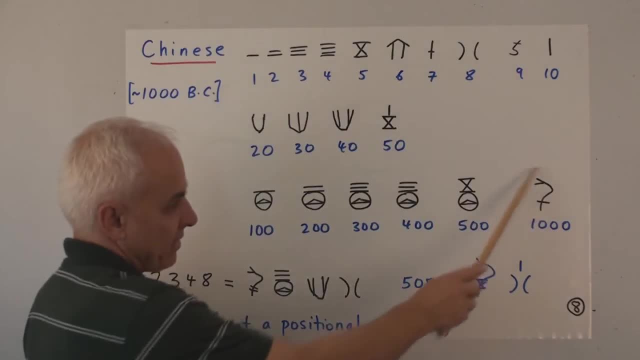 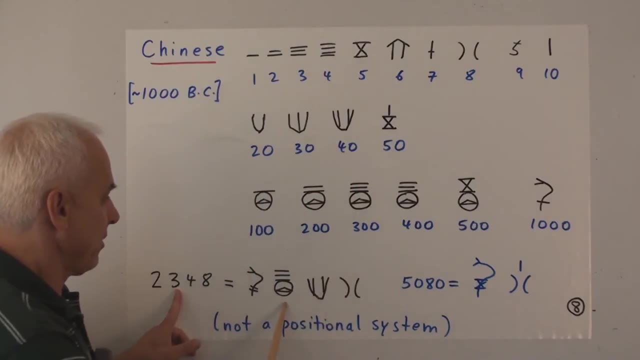 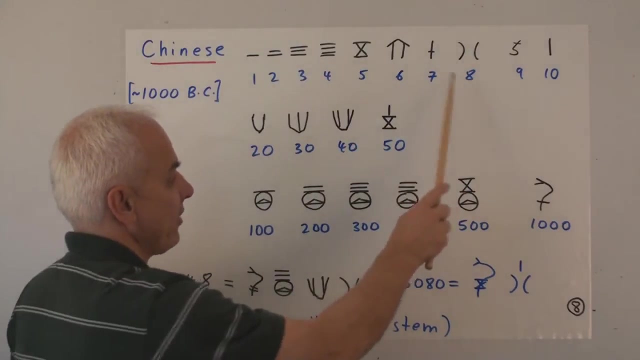 hundred and forty-eight would have been something like a thousand, with two bars in it to represent two thousand. The three hundred represented right there, The forty by that and the eight. that's one of our original ones. Now it might look like it's a positional system. 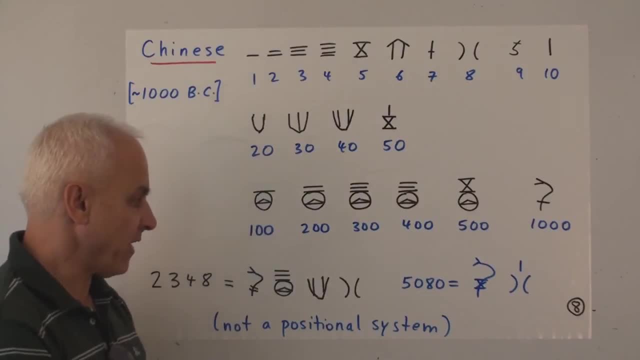 a lot like our Hindu-Arabic system, but it's not in fact So. if you look at five thousand and eighty, they would represent that by the symbol for five thousand, which is like the symbol for a thousand, with a five instead of a one on it, and 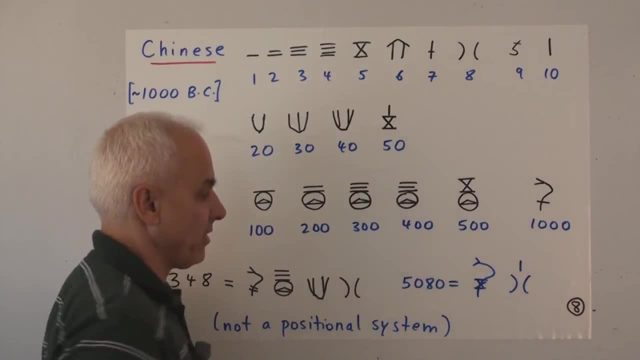 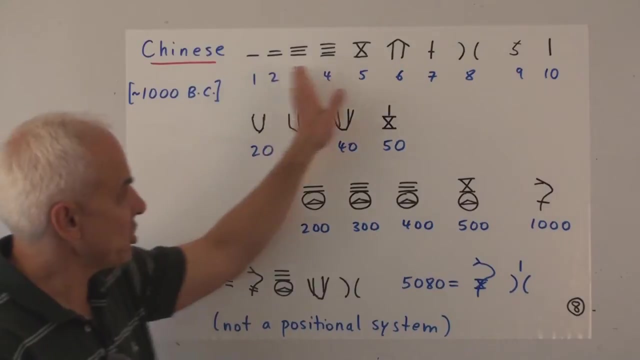 then the symbol for eighty, which was an eight, with this bar on top of it. But there was not a space here or anything like that to denote the zero hundredths, like we have, Just five thousand plus eighty. So it's not a positional system either. Nevertheless, it shares some key feature. 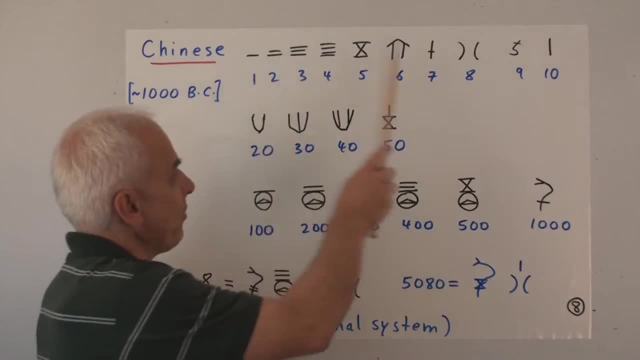 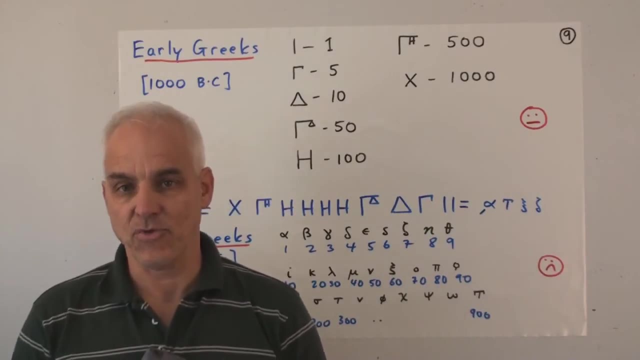 with the Hindu system, so that each of the numbers from one to nine gets a special symbol. The greatest mathematicians of the ancient world were the ancient Greeks, and they excelled in mathematics, And it's a little bit surprising that they were not able to make more progress with arithmetic and that they 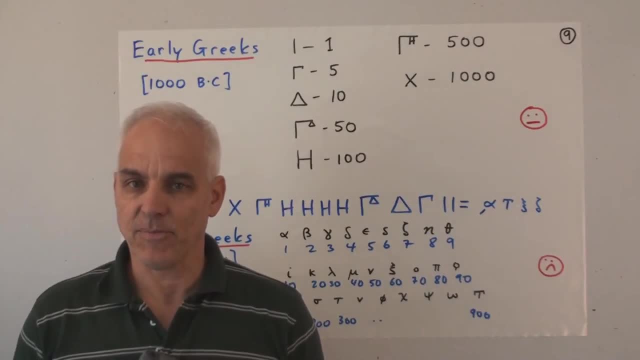 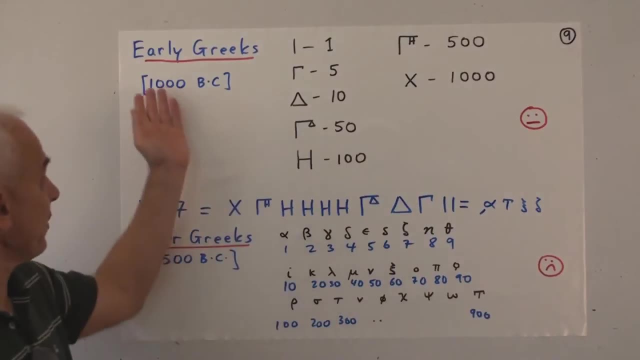 were not able to move to a better arithmetical system. There were kind of two periods in the Greek development in terms of arithmetical systems. There was sort of an early system and then a later system. The earlier system was a lot like the Roman. 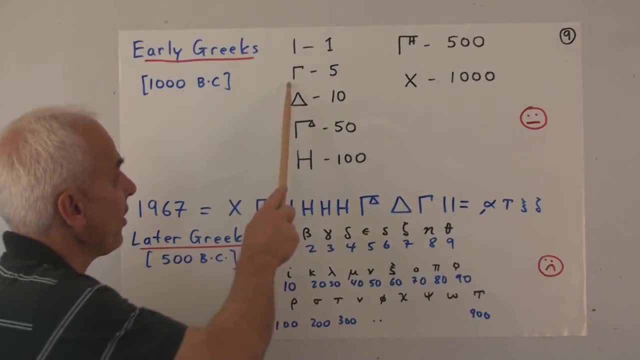 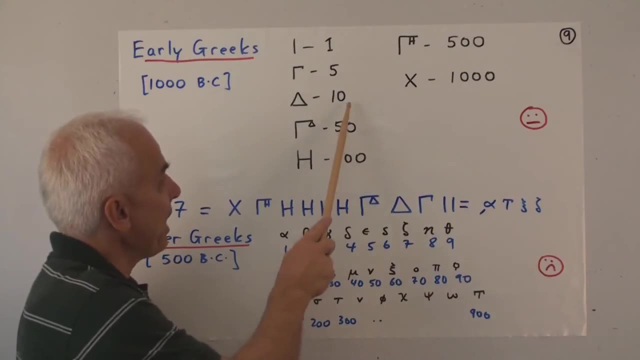 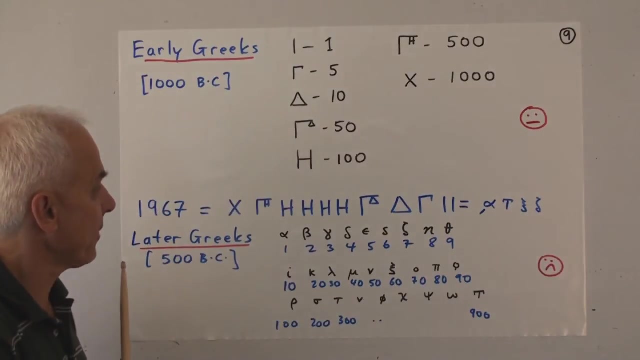 system. There was a stroke for a one, there was a lambda for a five, a triangle or delta for a ten, and then the fifty was a combination of the five and ten, sort of this five with a little triangle hanging from it. Hundred was H or something that looks like. 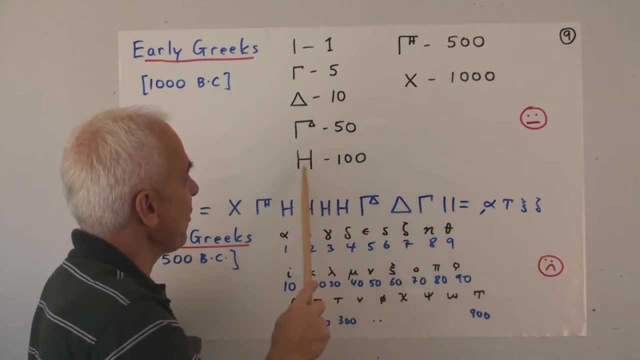 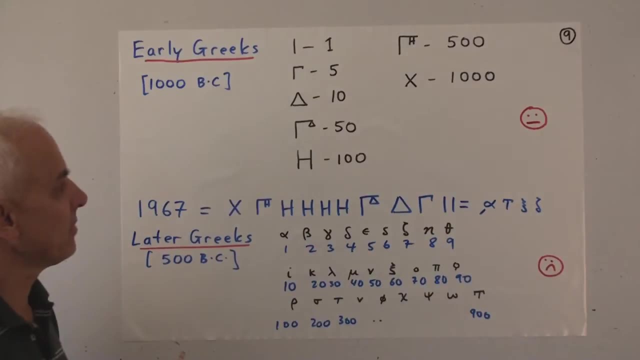 H, and then five hundred was again the symbol for five combined with the symbol for a hundred, in the same way that fifty was the five combined with ten, And thousand was X. Alright, so it's a lot like the Roman system. 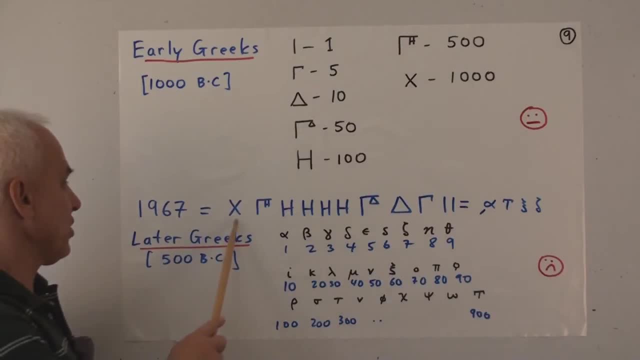 So 1967, that would be, there's the 1,000, reading left to right: 1,000.. This one here would be the 500, and then four more hundreds. So altogether this thing here would give us nine hundreds. 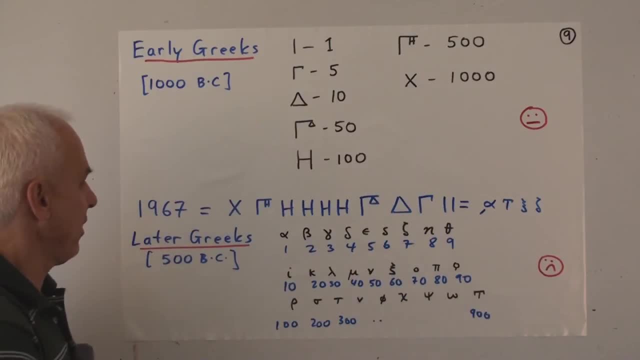 And there's 50, and there's 10,, so that gives us 60.. And there's five, and two ones give us seven. All right, sometime later they introduced a quite different idea, And here again the numbers 1,, 2,, 3,, 4, and so on all got separate symbols. 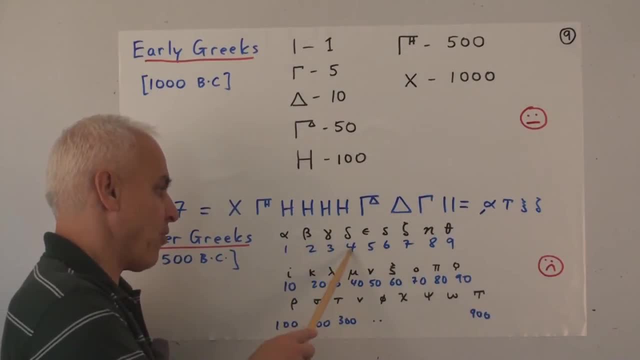 So 1 was alpha, 2 was beta, 3 was gamma, 4 was delta. You just recognize the Greek alphabet, Epsilon. okay, various other things whose names I probably can't say consistently, so I won't try. 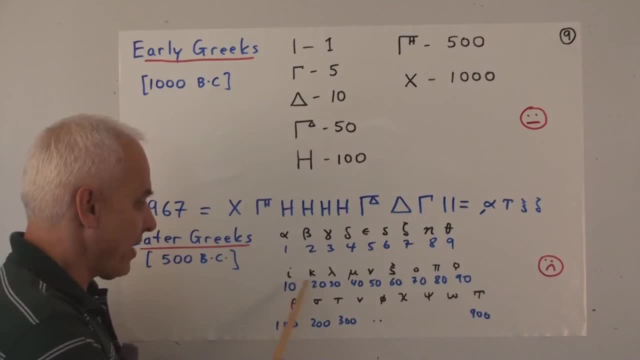 But once we get to 9 and 10, then also 20,, 30,, 40,, 50,, 60,, 70,, 80,, 90, all got separate letters. So the entire Greek alphabet here was employed to write down numbers. 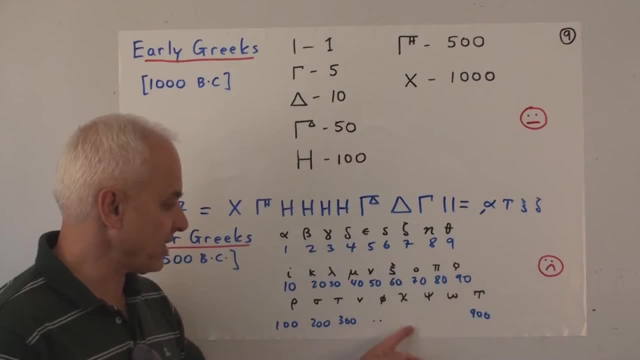 including 100,, 200,, 300,, 400,, 500,, 600,, 700,, 800, and 900.. So to write something like 1967 in this later thing, they would have first written 1,000.. 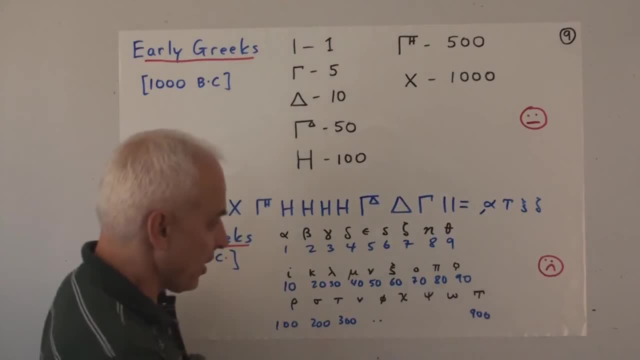 How is 1,000 written? Well, there's no 1,000 on this table. so what you do is you take 1, and you put a little stroke sort of in front of it, and that represents multiplying by 1,000.. 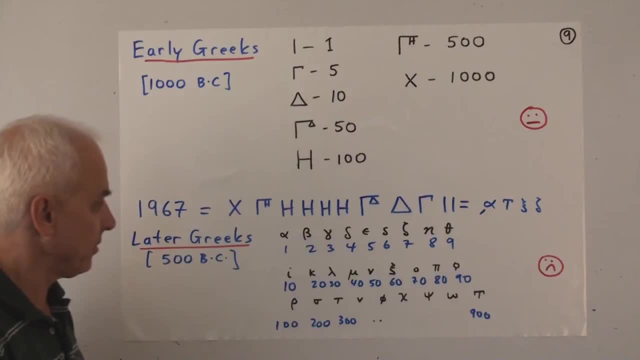 So that alpha with a stroke in front of it represents 1,000.. And then here we have 900, and 60,, here 60,- this is beta- and 7. So it's a relatively efficient way of writing numbers. 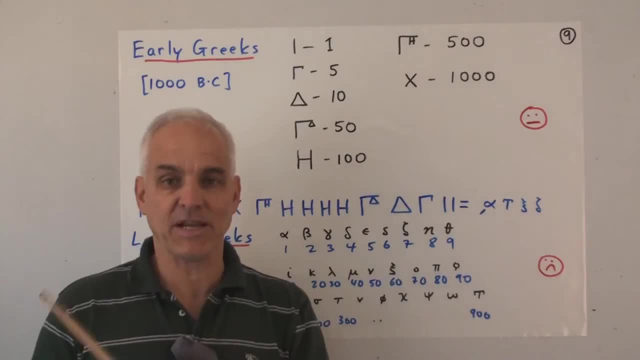 but the price that you pay for having an efficient way of representing the numbers is that the operations become difficult to do. So you can imagine what a headache it would have been for schoolchildren to learn how to multiply numbers in this system. Well, they probably wouldn't have learned. 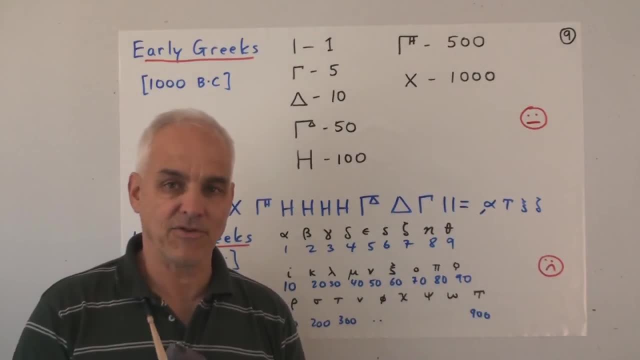 It would be only very special scribes and scholars that would be able to multiply numbers in this system is my guess. Now there's one of the ancient civilizations that we haven't talked about, and I'm not going to talk about it today, because it's the most sophisticated one. 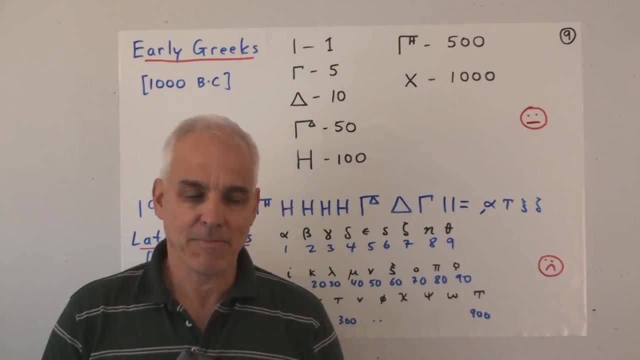 It's the Babylonian system. In fact it's the earliest one. The Babylonian system is quite different from all the others and it's actually pretty interesting, But it's not something that is easy to describe until we build up a little bit more mathematical experience. 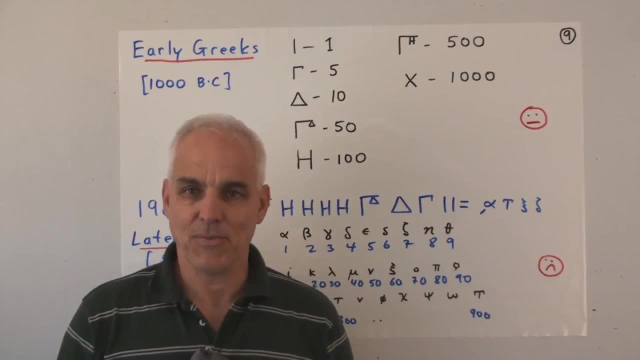 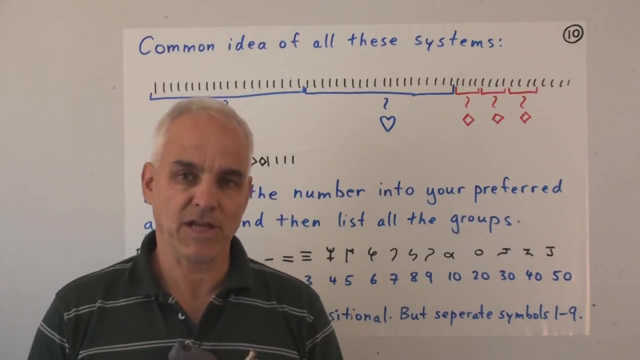 So sometime later we'll come back to the Babylonians and I'll tell you what their number system was like. All of the systems that we're looking at have a basic common orientation, And it's the orientation that we started out with, the sort of common sense idea. 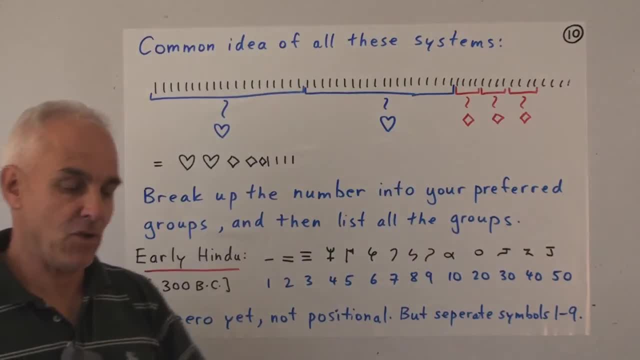 You have a big string of ones and you want to describe that more efficiently. So you decide on various groupings that you give some names, and then you look in the string and peel off the biggest groupings that you can. That's in real time. 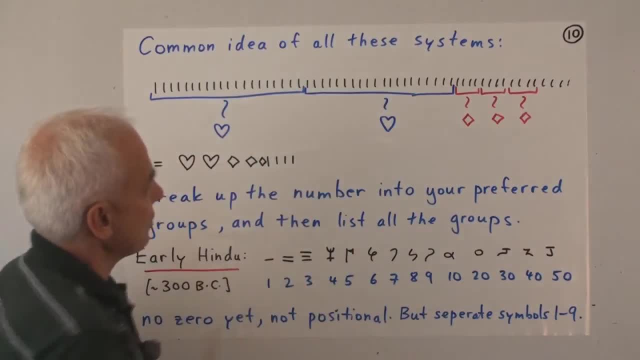 That's in your system. So here, just to give you an example, suppose I had a grouping called a heart which in fact has 20.. So then I would say: aha, that's one heart, That's a set of 20.. 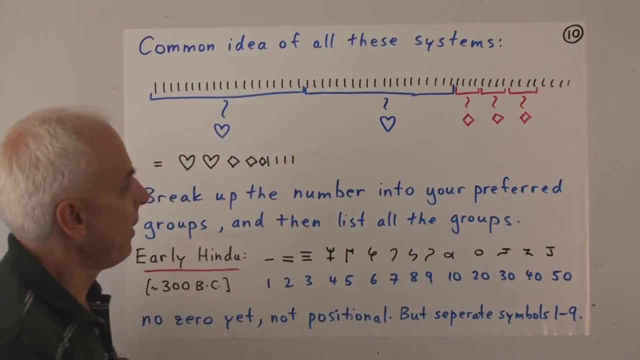 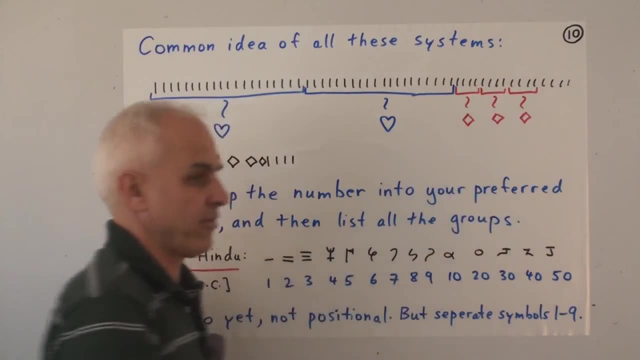 Here's another set of 20.. So I have two hearts and then maybe a collection called a diamond, another diamond, another diamond and then four ones. Then we would represent this number by just listing the groups one after the other. 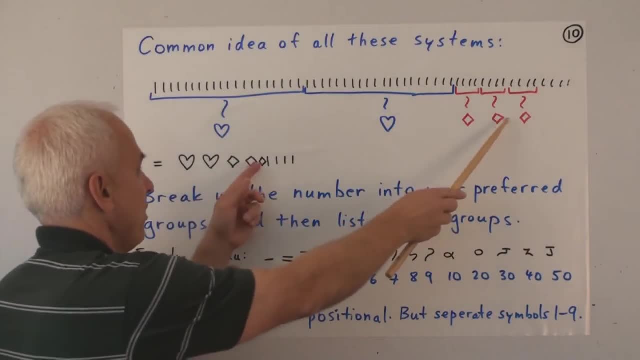 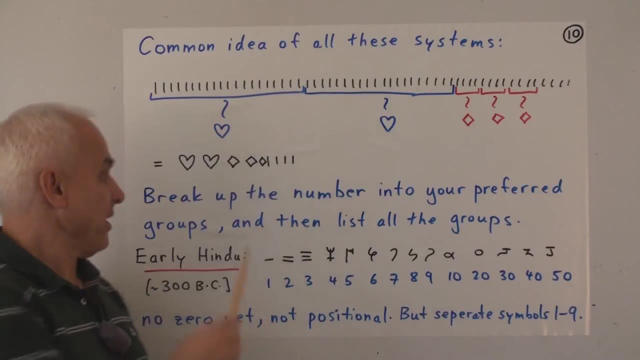 There's the first heart, then the next heart, and then a diamond, diamond, diamond, one, one, one, one, And we could go back to the original number by replacing the symbols with a whole bunch of ones, depending on what the symbol was. 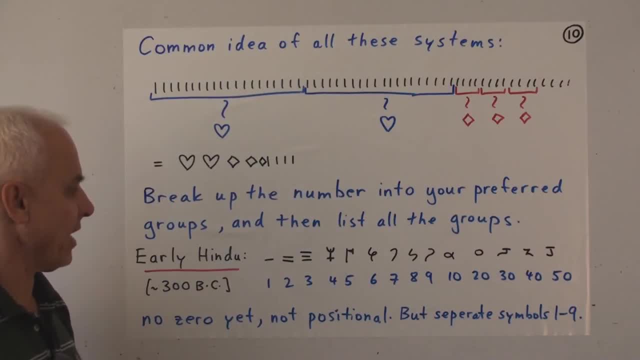 So it's a very common idea. Now, the civilization that we haven't talked about is the Hindu, The early Hindu system. And here is their, the symbols they had. They also had symbols for the numbers 1 through 9.. And if you look at them, 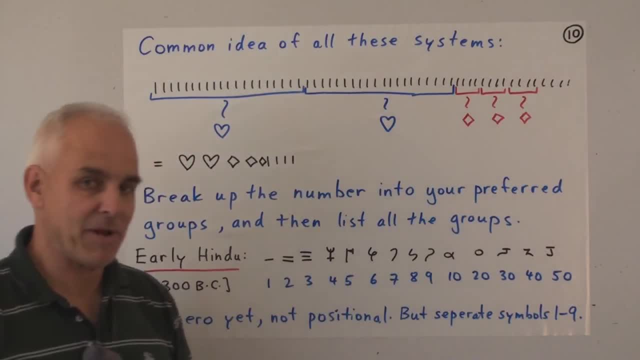 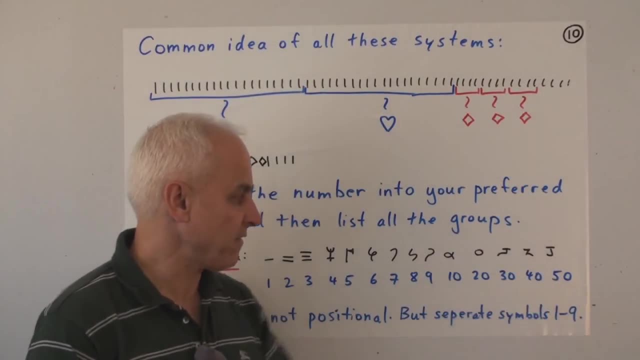 you can start seeing, I hope, something getting a little bit close to our numerals. They had a special symbol for 10,, 20,, 30,, 40, and 50. They did not have a zero at this point.